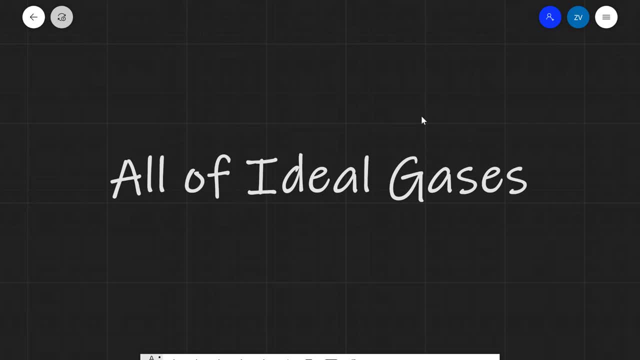 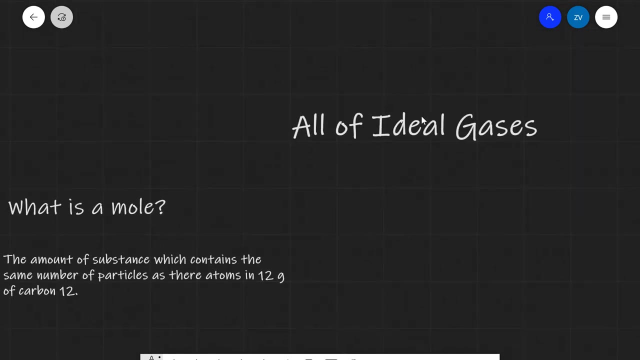 Today we're going to be revising thermophysics again. So this is part two: all of ideal gases. If you're looking for part one, which is the rest of thermophysics, please have a look at a link in the description of this video. Well, let's get started. The first aspect of revision. 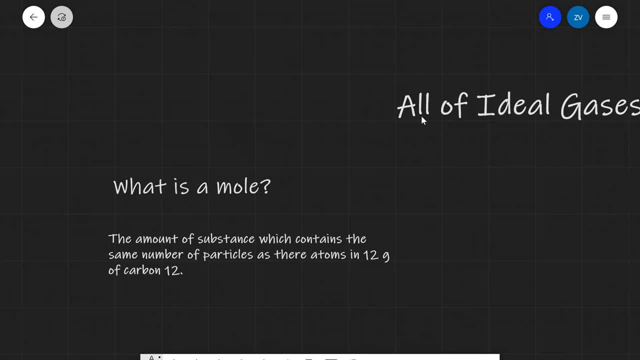 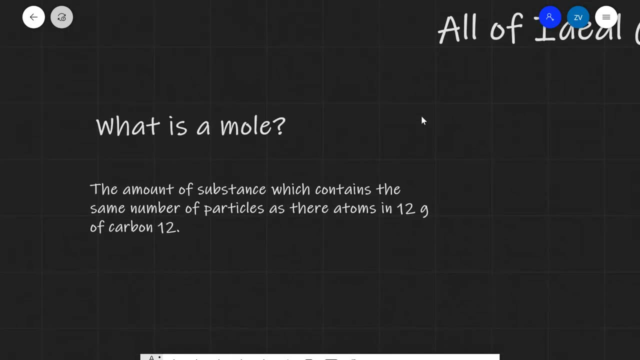 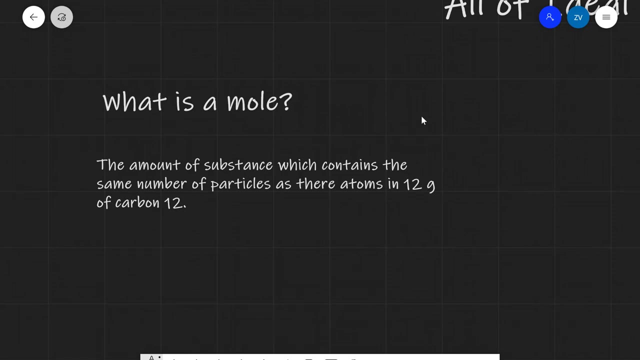 for ideal gases would be. what is a mole? Now? contrary to popular belief, this is not a small creature that lives on the ground, but a mole is the amount of substance which contains the same number of particles as there are atoms in 12 grams of carbon-12.. And this number is 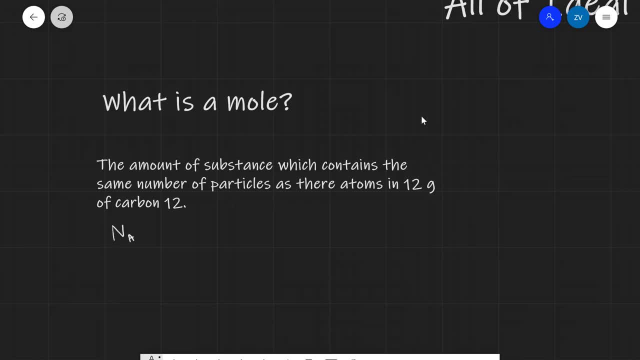 Avogadro's number- So let's call that an A, which is about 6.02 multiplied by 10, to the power of 23 particles. So, for instance, we could have one mole of water, one mole of acid and one mole of carbon-12.. So, for example, we could have one mole of nitrogen. 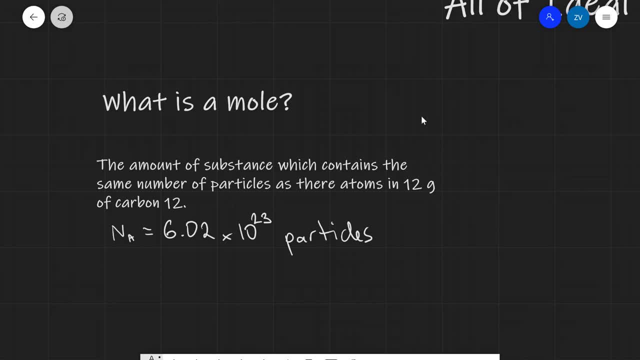 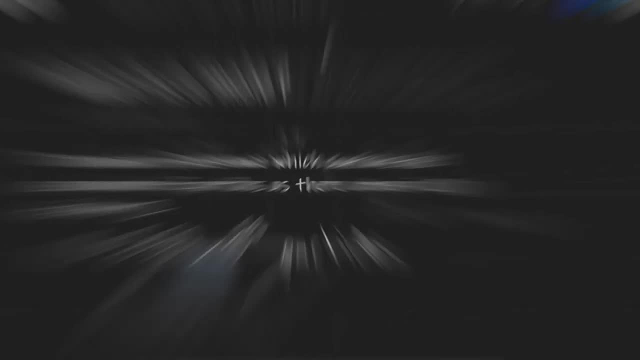 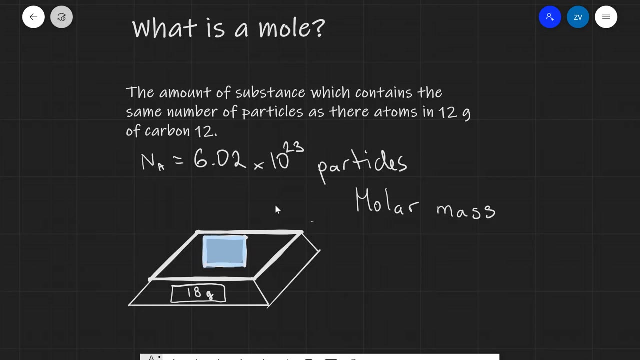 and one mole of oxygen. So, for example, we could have one mole of nitrogen and one mole of oxygen of metal, etc. and each of them will contain the same number of particles: 6.02 times 10 to the power of 23. okay, next up is the concept of molar mass. the molar mass will actually allow us to know. 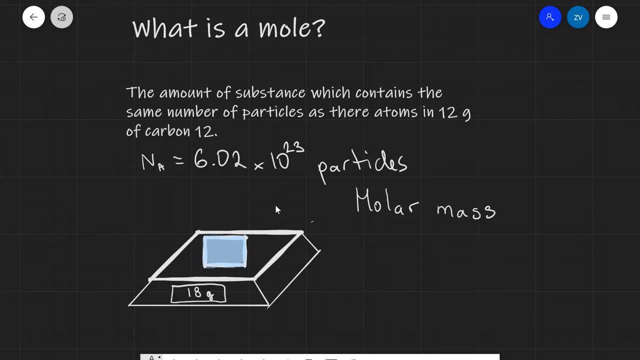 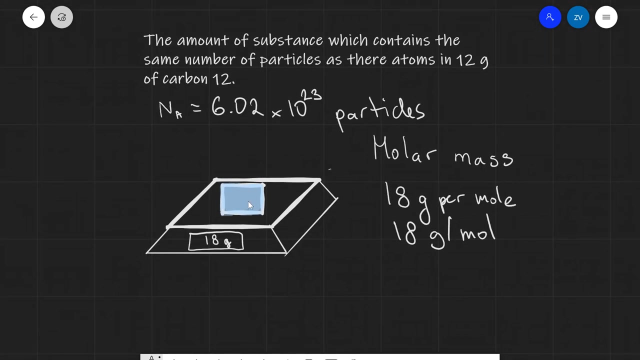 how much does a mole out of a particular substance weigh, for instance the molar mass of water? let's just say the molar mass of water is 18 grams per mole, which is also commonly written as 18 grams divided by moles. okay, well, this means that, essentially, if we had some water and if we 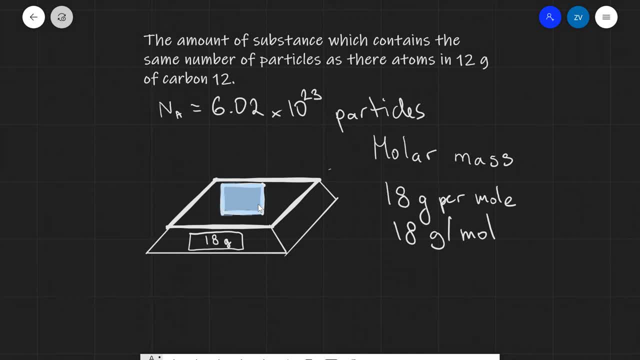 had one more particles. so remember one more particles is Avogadro's number. so if we have 18 grams of water, exactly because that's the molar mass, the number of particles contained within the container will be Avogadro's number, or 6.02 times 10 to the power of 23. 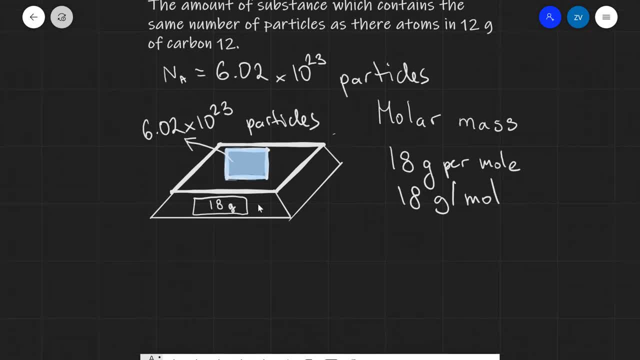 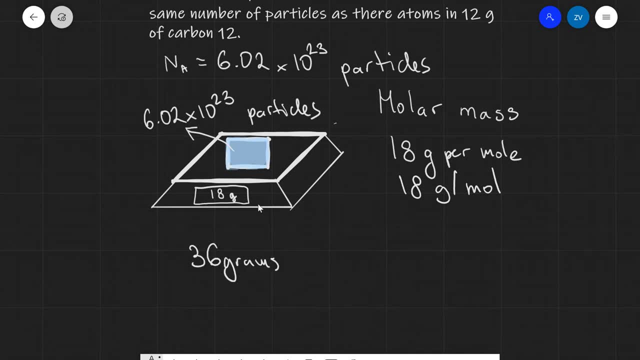 particles. now, if we were to have, let's say, 18 times twice is 36 grams of water, we would have double that. so we would have about 12 or 4 times 10 to the power of 23, which is about 1.204 times 10 to the power of 24 particles. 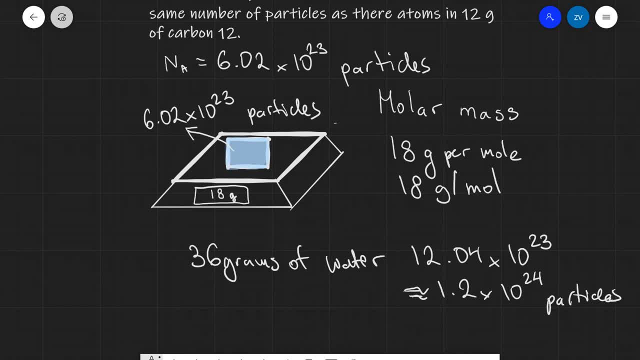 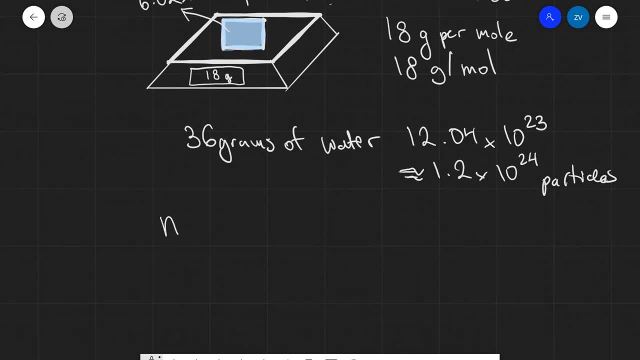 and we can generalize this idea in a couple of different equations. our first equation is that the number of moles- I'm just going to write this as a word equation for once- the number of moles typically given, n, is equal to your mass measured in grams or kilograms, depending on the data that we're given and that will be. 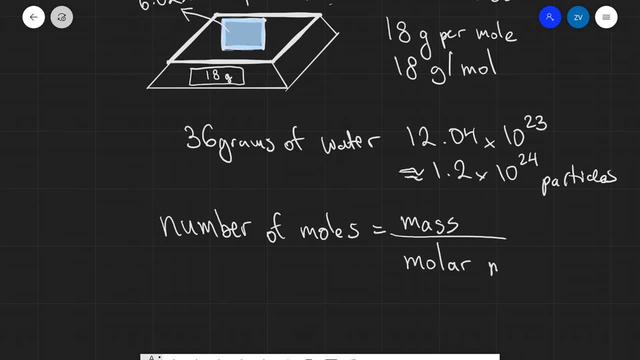 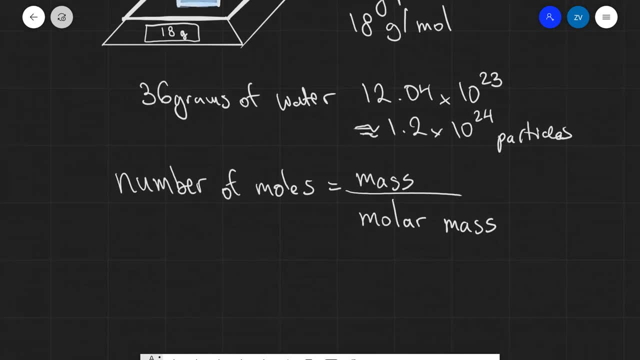 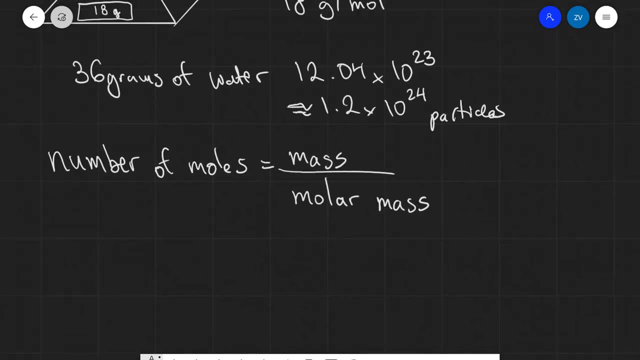 divided by the molar mass. so the way I normally remember it is M over MM, mass over molar mass. this equation is not typically given in your formula sheet and we can also kind of work it out just by thinking about units. if we think about it right here in the top, let's say we 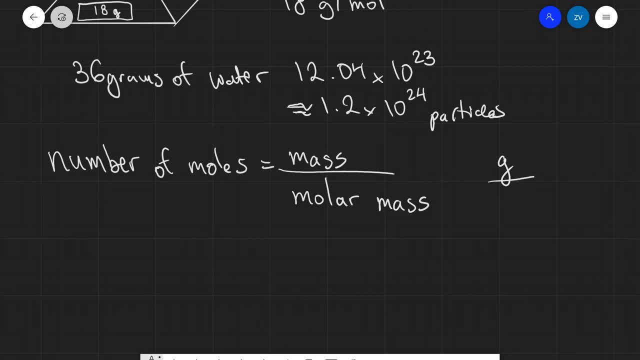 have grams or kilograms and then we're dividing these by 0.5 grams of limit and then we're dividing it by the molar mass. if we think about it right here in the top, let's say we have grams or kilograms and then we're dividing it by the number of moles, then we can divide. 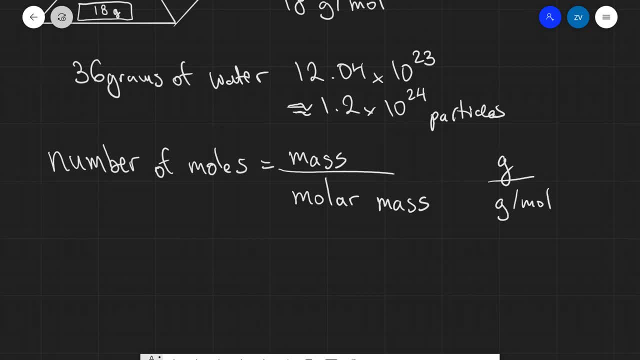 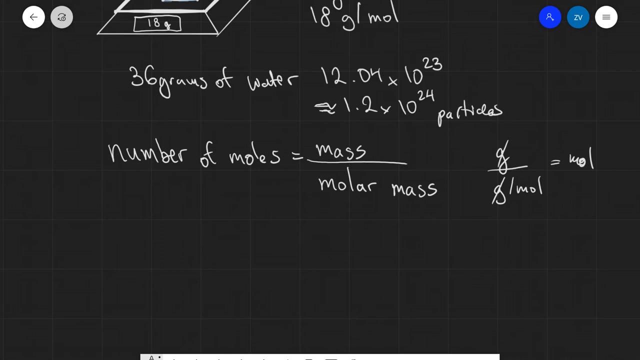 that by grams per mole, which is equal to 1 over 1 over mole, which of course is just gives us moles, so a number of moles, is that once we have the number of moles, what we can actually do is work out the number of particles. number of individual. 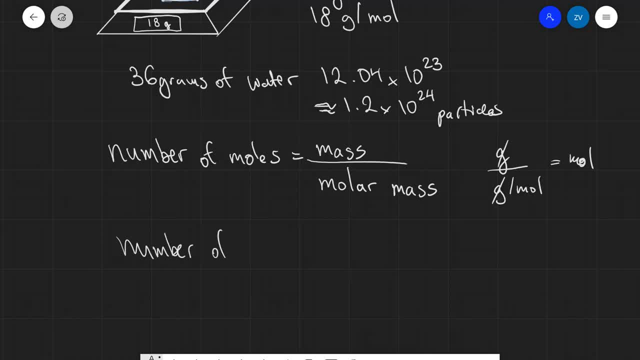 particles, so number of particles which will just be equal to our number of moles, which can writers? and this, actually, let's be consistent, and let's write as number of moles multiplied by Avogadro's number, which is n a 6.02 times. 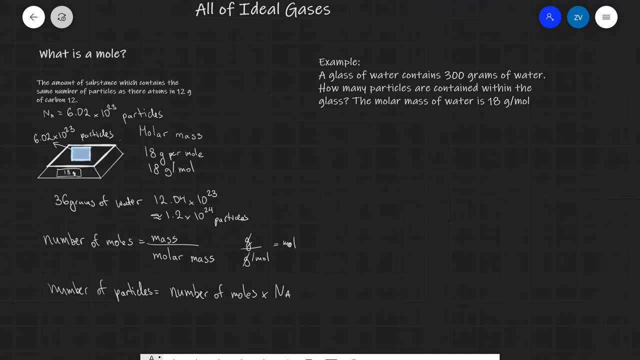 10 to the power of 23. okay, well, let's have a look at a little example. over here we have a glass of water containing 300 grams of water. how many particles are contained within the class? the molar mass of water is 18 grams per. 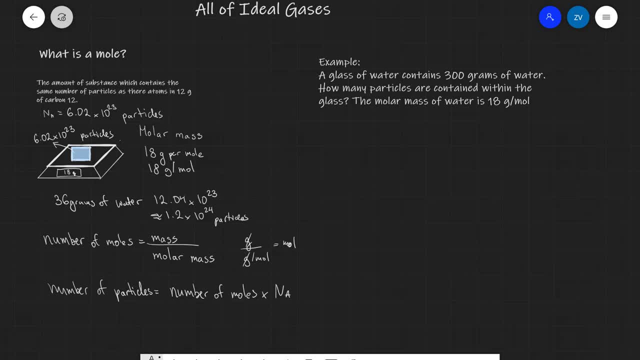 mole. well, because we're curious, we can start thinking about how many particles are we actually holding when we have a glass of water, if the water weighs, let's say, 300 grams. first off, we need to work out the number of moles. so, remember, and the number of moles is M of mm, so it's gonna be mass of a molar mass, so that's. 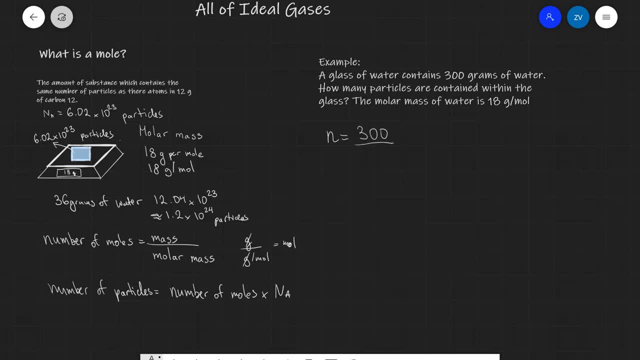 going to be the number of moles. so that's going to be the number of moles going to be 300 grams divided by 18 grams per mole, which is going to give us approximately sixteen point six, seven moles, and what I'm going to do. 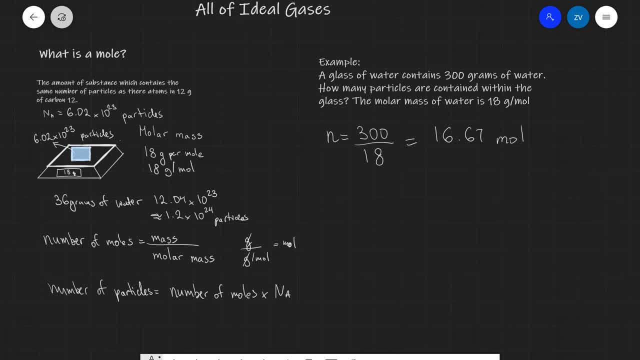 afterwards is I'm going to just multiply that number by Avogadro's number to work out the number of particles, because, remember, one of these moles is actually equal to an Avogadro's number of particles. so the total number of moles is the total number of particles. let's call that capital N. so remember, typically in 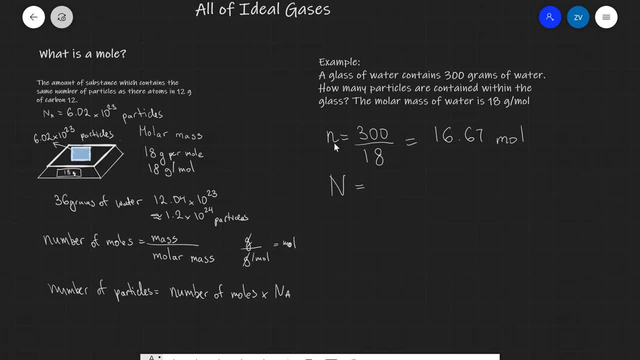 physics s lowercase n is the number of moles. capital N is the number of particles. so the number of particles will then be equal to just sixteen point six, seven multiplied by six point oh, two times ten, to the power of 23. never put that into a scientific calculator. 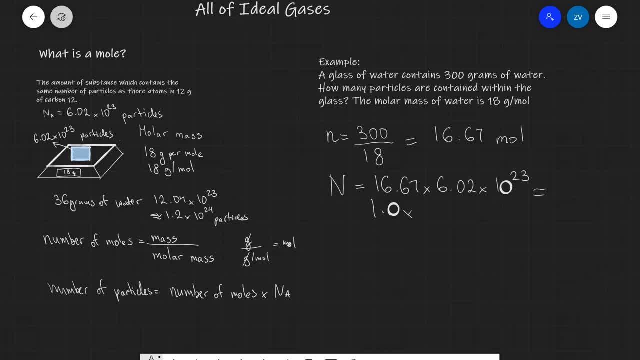 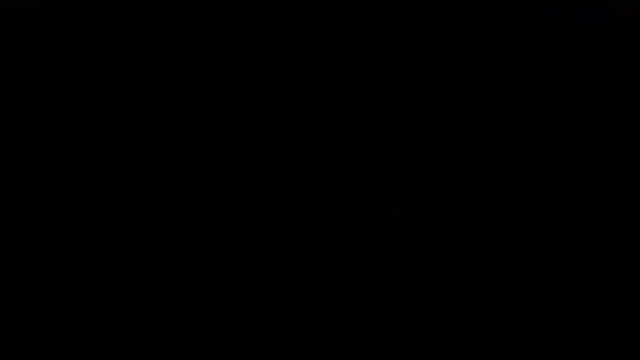 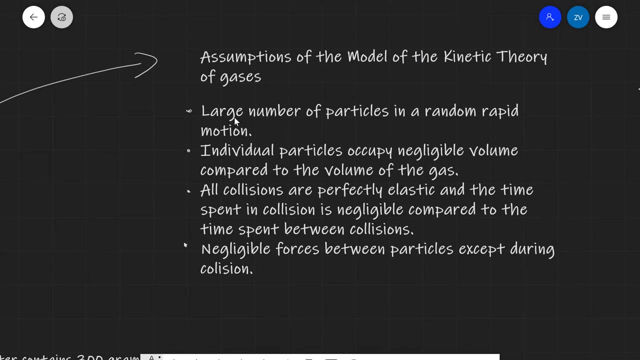 we are going to get about one point zero times ten to the power of 25 individual particles. okay, now that we've had a look at the number of moles, let's look at ideal gases in a little bit more detail. we can think about ideal gases using the: 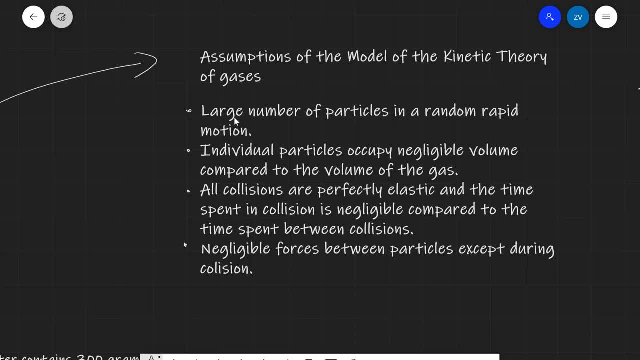 kinetic theory model of the gases that tells us there are large number of particles not wrapped, random rapid motion, and this is actually a very good example of that. so this is actually the first of the assumptions of this model, which would need to be remembered before an exam. so this is our first assumption. 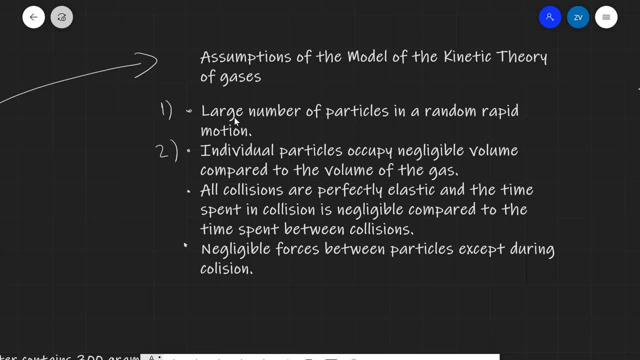 our second assumption tells us that the individual particles occupy negligible volume compared to the volume of the gas. in the words, the particles are very, very small. three: all collisions are perfectly elastic. remember, in a perfectly elastic collision kinetic energy is conserved and the time spent as collision in 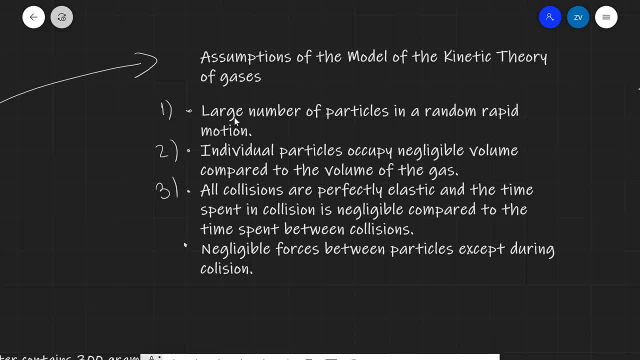 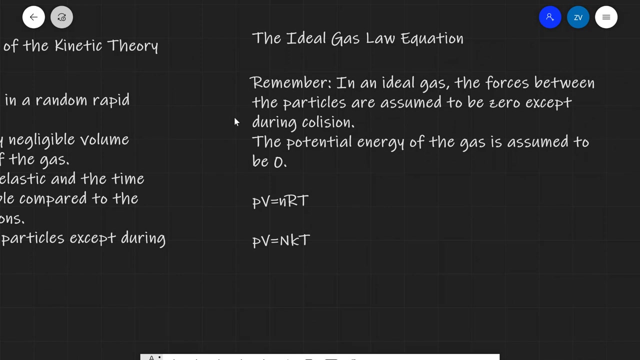 a collision is negligible compared to the time spent between collisions. our fourth assumption is that there negligible forces between the particles except during collision. so this means the particles are basically not attracting each other unless or not interacting via any of the forces, unless they're colliding. well, this leads us to the ideal gas law equation, and just a. 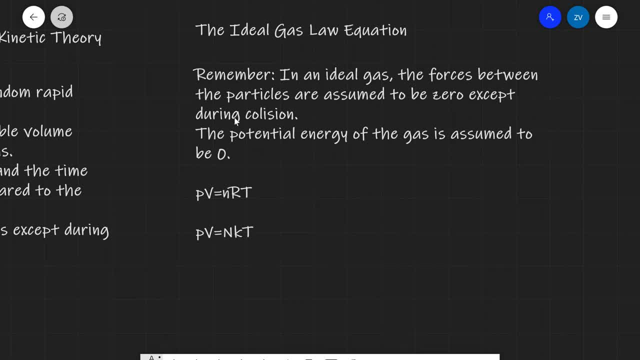 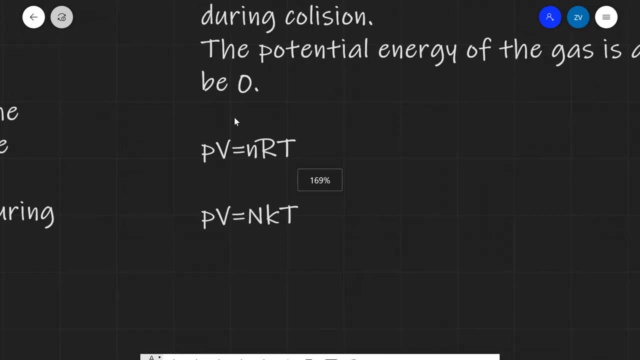 couple of really important points to remember as well from the previous slide. as we said, an ideal gas. the forces between the particles are assumed to be zero, except during a collision. because of that, the potential energy of the gas is also assumed to be zero. well, there are two equations which govern the behavior. 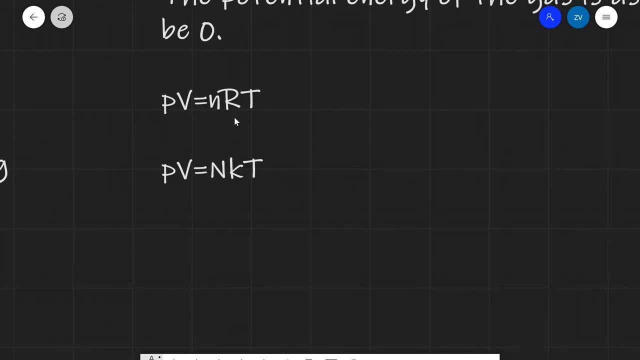 of ideal gases, and they're very, very important. PV is equal to nRT and PV is equal to n times K times T. they're essentially the same equation. P stands for pressure, V stands for volume. now in this equation the lowercase n is the number of moles, so we can write that in the number of. 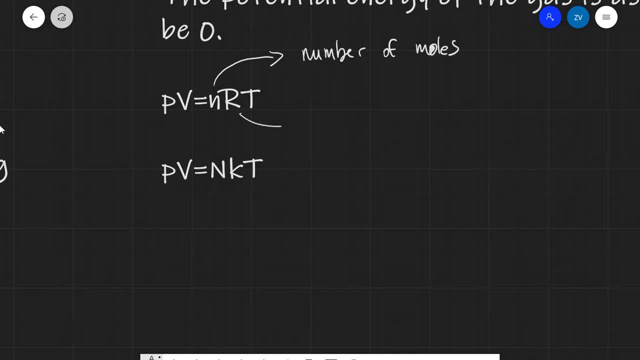 moles R. here is the gas constant or the gas law constant, which is just approximately equal to 8.31. so we can just write that in 8.31 and T is the temperature in Kelvin. so this is very, very important. quite a typical mistake would be to have 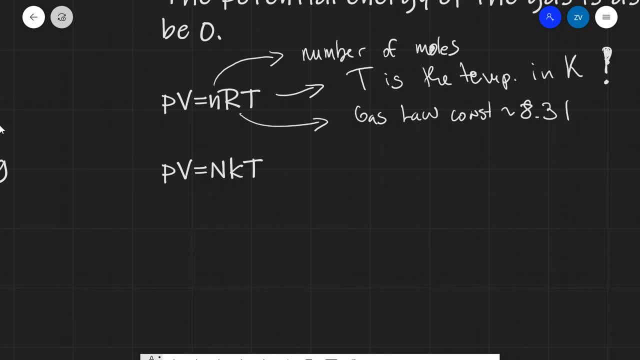 a problem in which the temperature is given in degrees Celsius. remember, we need to convert that to Kelvin. the lower equation is basically the same equation. however, rather than the number of moles, we just converted to a number of particles. so the uppercase and in this case is the number of particles and the 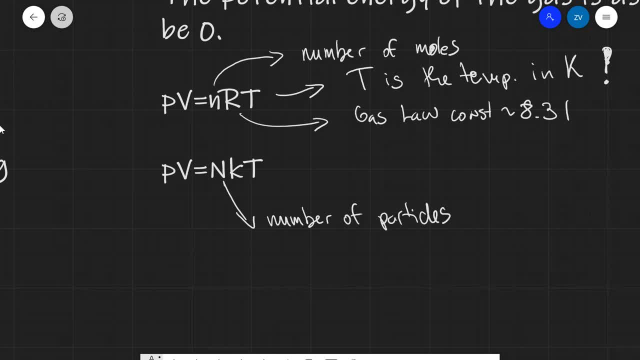 economic force is the percentage ofOOOOOOOOOOOOOOOOOOOOOOOOOOOOOOOOOOOOOOOOOOOOOOOOOOOOOOOO. copies. subtle K: sorrow cry. now, on what are we shadows? so we can quickly prepare the. 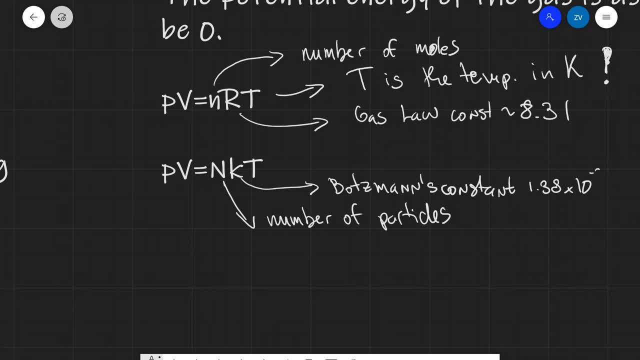 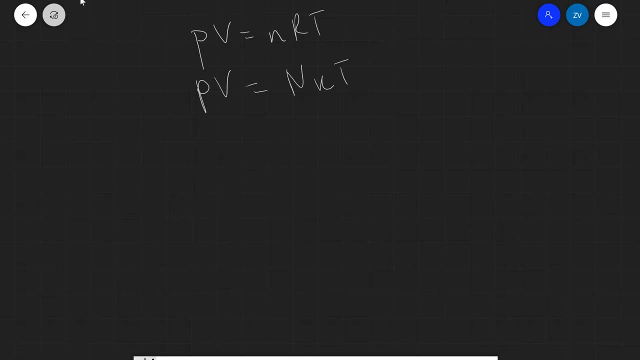 mass. we're gonna write down about the mole mass so you can see that we have by the, by your pole, the number of moles being equal to, ah, Kelvin. Now, looking at those two equations, there's one more factor that I really like to. 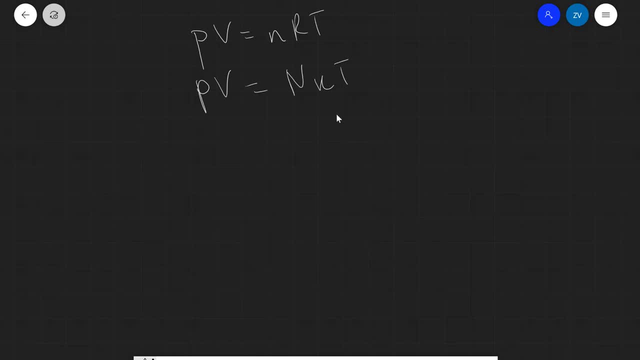 mention, and that is about Boltzmann's constant K, Because PV is equal to nRT and PV is equal to nK times T. then what we can do- let me just make this a little bit more legible- that's T here. 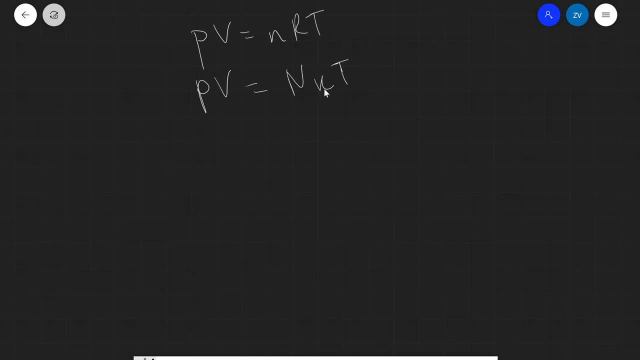 what we can do is essentially set those parts of the equation equal to one another. nR will have to equal n multiplied by K. Well, let's just rearrange for K. K will be equal to nR divided by the number of particles. Once again, in this equation, lowercase n is the number of moles, uppercase n is: 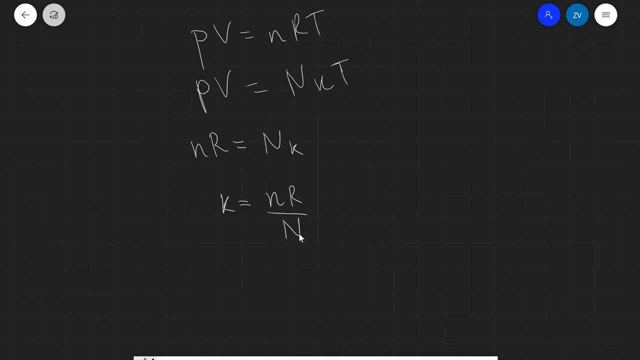 the number of particles. But how are they related? Remember, the number of particles. n is equal to the number of moles multiplied by Avogadro's number 6. About 6 times the integral power of 23.. Okay, well, let's just sub that in here, and what we're? 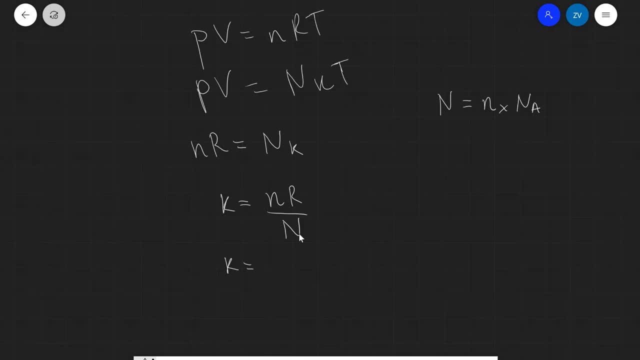 going to get is that Boltzmann's constant K will be equal to nR over n times Avogadro's number. Those guys are going to cancel and we're going to find that Boltzmann's constant is equal to the. 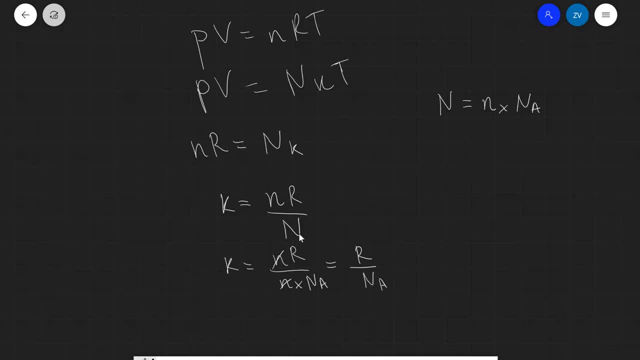 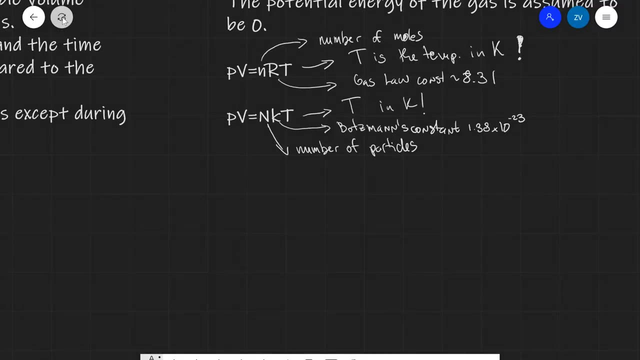 gas flow constant divided by Avogadro's number. Now let's have a think about the ideal gas behavior if let's say the temperature is constant. So first off let's look at what will become known as Boyle's law after we set the temperature to be a constant. So let's say 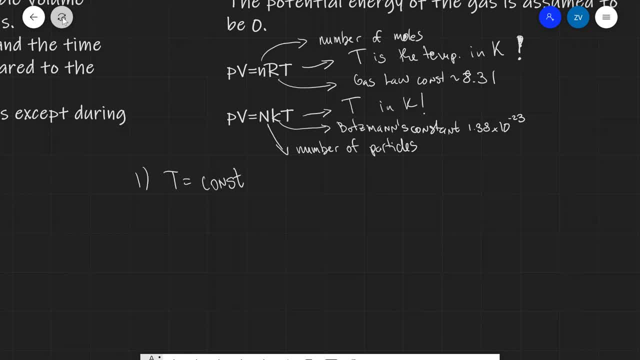 that our temperature is equal to a constant In practice. for instance, we could be increasing the pressure by decreasing the volume with a pump very, very slowly to try and keep the temperature constant, for instance. This would be a physical scenario for this. But if the temperature is a constant, because PV is, 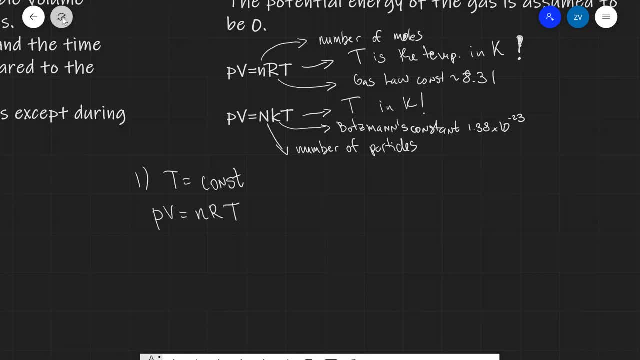 equal to nRT, and let's say that the temperature is constant for the fixed volume, so for a fixed amount of gas, then the pressure could be varied, the volume could be varied and the number of moles, which is the constant R, is just. 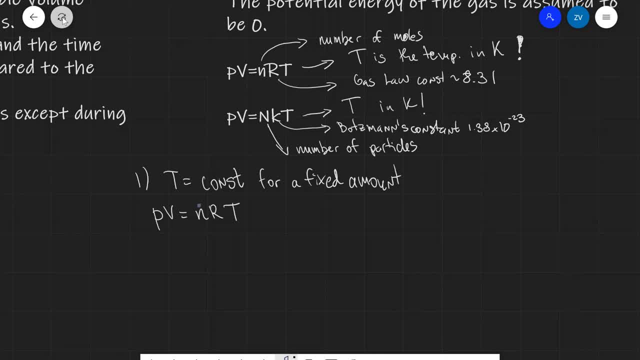 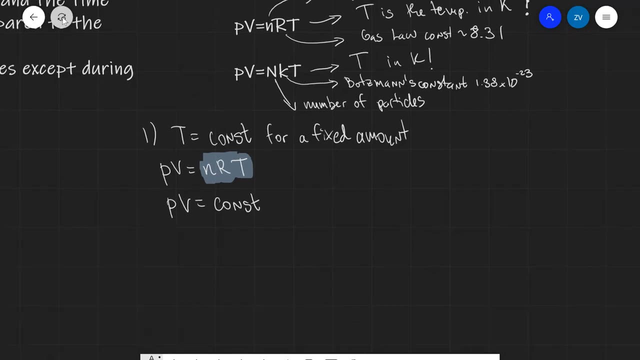 constant, then the temperature is a constant. so if that's the case, the whole of the right hand side that I'm actually highlighting now is a constant. so P times V will be a constant, which would mean that P is going to be a constant divided by V, which would mean that P is proportional to 1 over V. in other words, 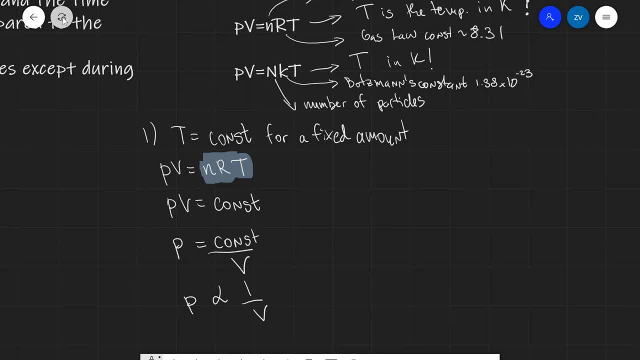 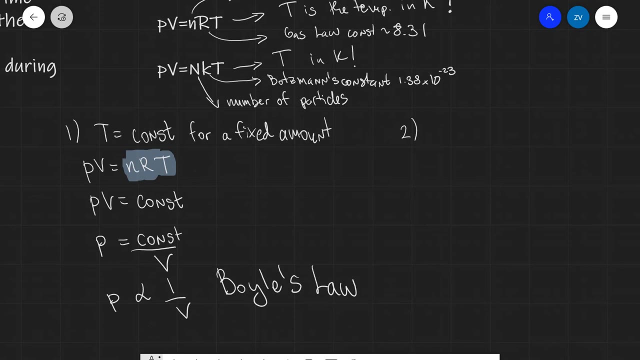 the pressure is inversely proportional to the volume at a constant temperature for a fixed amount of gas, and this statement is known as Boyle's law. now let's think about what would happen if we kept V to be a constant. so keep the volume constant. maybe it's a metal container that we're dealing with, or a 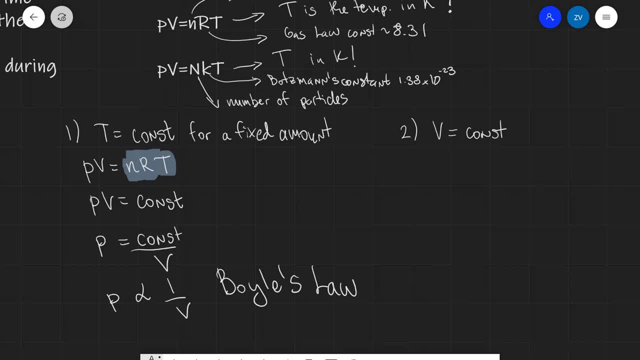 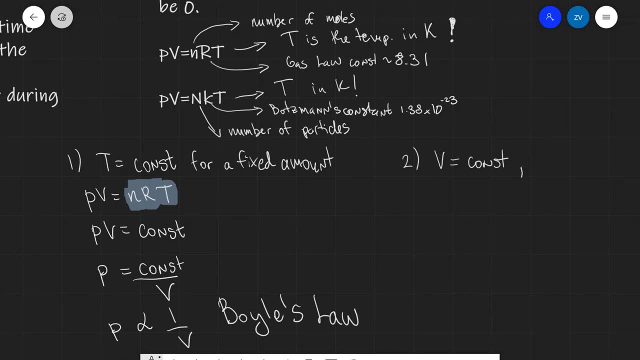 glass container or something which doesn't really change its volume. you, and let's say that also the amount of substance is constant, so n is equal to a constant, so no gas is leaking out of our container. well, if that's the case, well then that would mean that P will be- let's just rearrange- PV is equal to nRT, so I'm 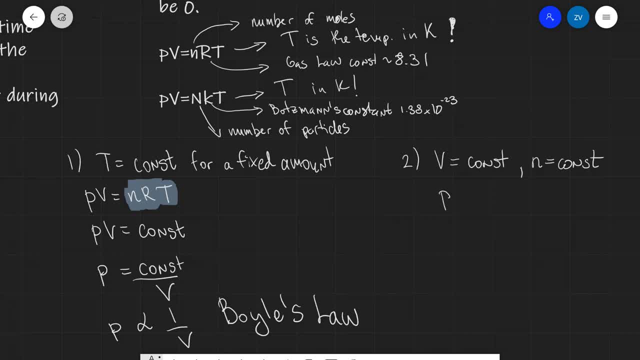 going to start off with. PV is equal to nRT here. so PV is equal to nRT, and because V is a constant, now I am going to just rearrange P. so I'm going to say that P is going to equal to nR divided by V times T. well, have a look at that. n is a constant, R is a. 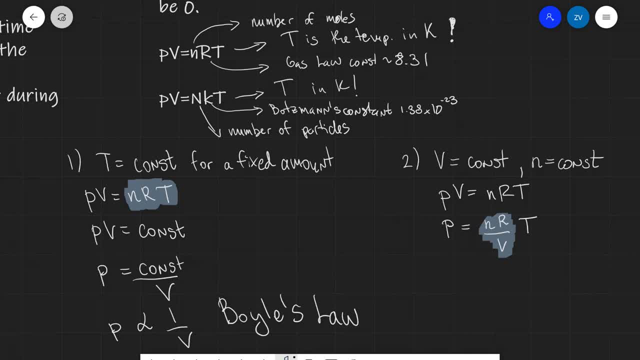 constant and V is a constant. so this whole highlighted area is equal to a constant. so this means that the pressure is equal to some constant multiplying by T, which means that the pressure is directly proportional to temperature for a fixed mass of a gas, if the volume is kept constant, this is known as our. 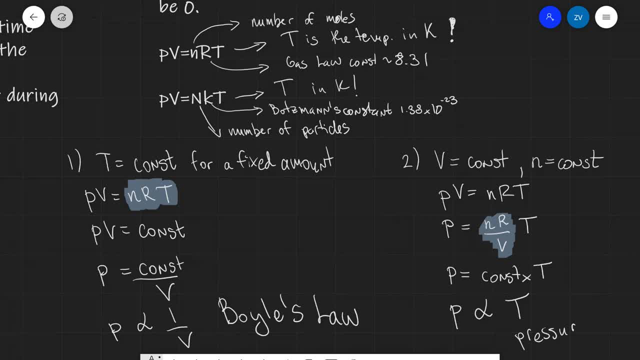 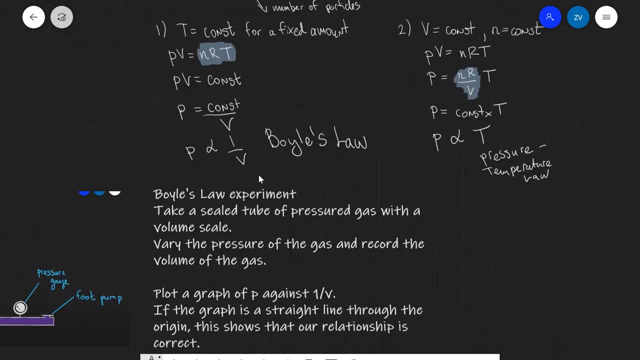 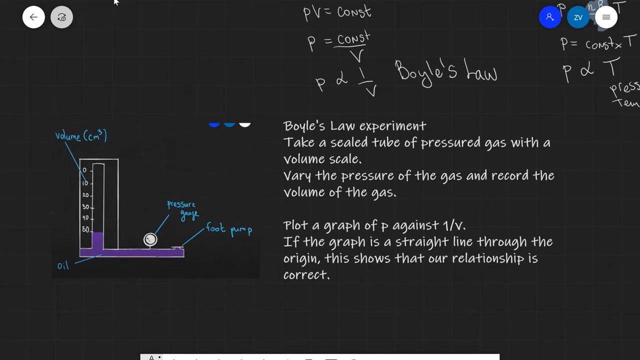 pressure law so you can write it down as our pressure temperature law. now that we have had a good look at our two laws, let's have a look at an experiment for Boyle's law. so the way we're going to do this experiment to prove that Boyle's law is correct: we're going to take a sealed tube of a pressured 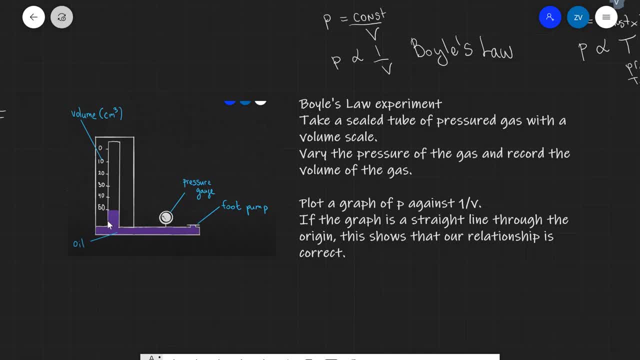 gas with a volume scale. typically this is filled with oil as well, at least partially with oil. so we're going to vary the pressure of the gas and we're going to do that with a foot pump or just a regular pump, and we're going to have a pressure gauge and we also have a volume scaled. we're going 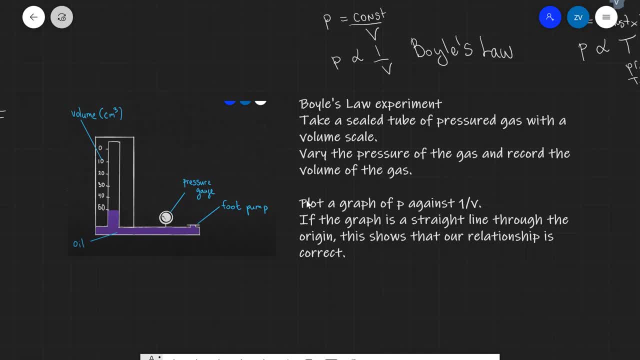 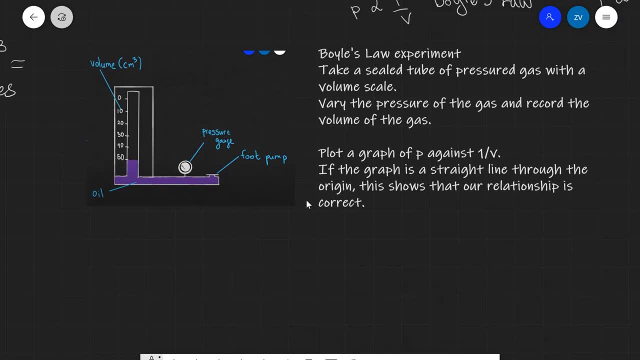 to measure the pressure with a pressure sensor or a pressure gauge once again. so it might be worth just adding a list of measurements. so let's do that really quickly. so I'm gonna say measurements and say the volume and the scale, the tube and our pressure with the pressure gauge or a sensor as well, if that's available. afterwards we're going to plot. 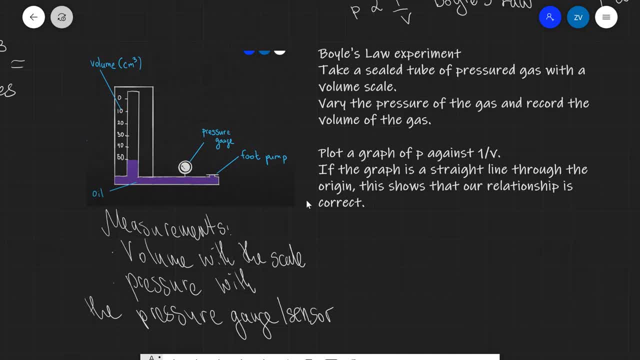 a graph of the pressure against 1 over V and if the graph is a straight line for the origin, this shows that our relationship is correct. remember, if we have a graph of the pressure against one of the volume, this will be expecting a straight line relationship. why is that? remember? 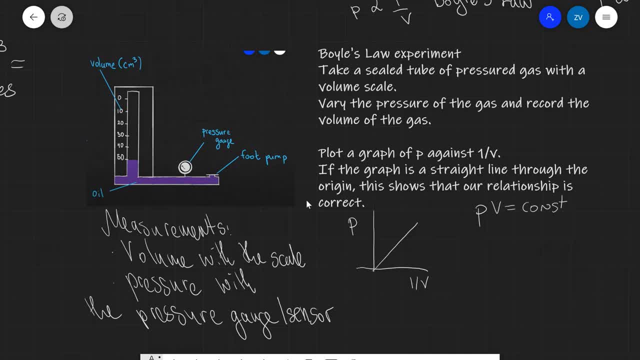 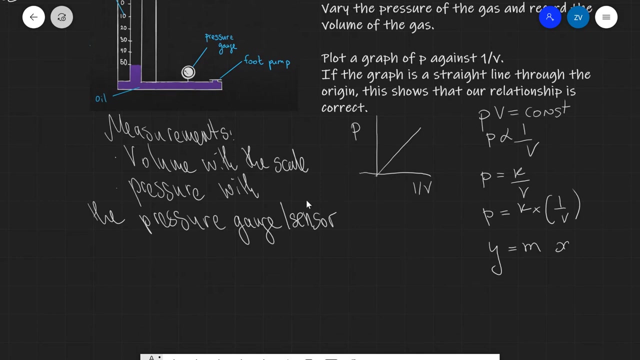 P times V is equal to a constant, which means that P is proportional to 1 over V. so P will be equal to some constant. let's call that K divided by V, which means that P is equal to K times 1 over V. now, just in the name I'm going to write, Y is equal to a max plus C. I'm gonna add a plus zero. 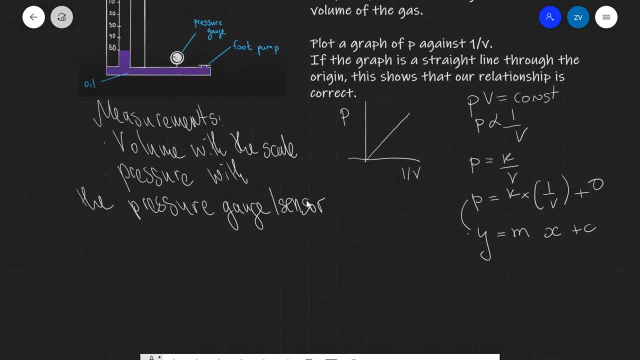 here. so if P is uncertainty, y-axis, if 1 over V is on the x-axis, what's left for our gradient is is our constant. so in this case our gradient be equal to our constant, which is actually equal to nRT. and that is because PV is equal to nRT in general. so we could, if 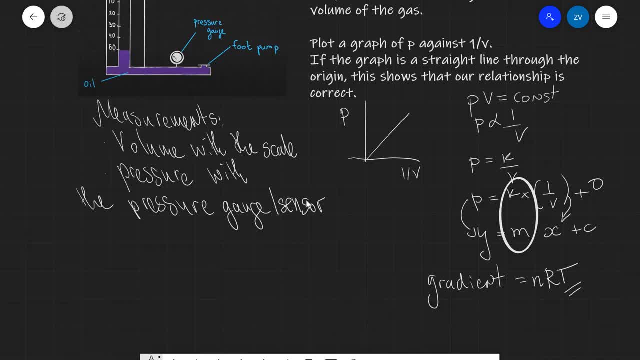 we were given the temperature, for instance, from the gradient of this, of this graph, we could work out our, our, our number of moles, for instance, or if we're given both of those, we could work out the constant R if we didn't know it, etc. so this is a really, really important experiment. now, how could we make this? 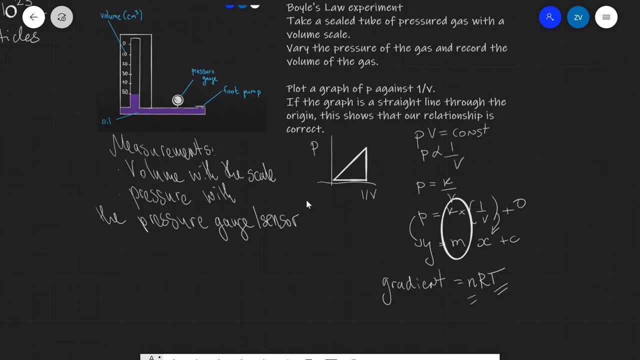 this experiment better. well, we need to ensure that the temperature is constant, and this is really important, so I'm just going to add that in in here, and this is really important, so I'm just going to add that in in here. so what I'm going to say is: vary the pressure slowly, so vary the pressure. 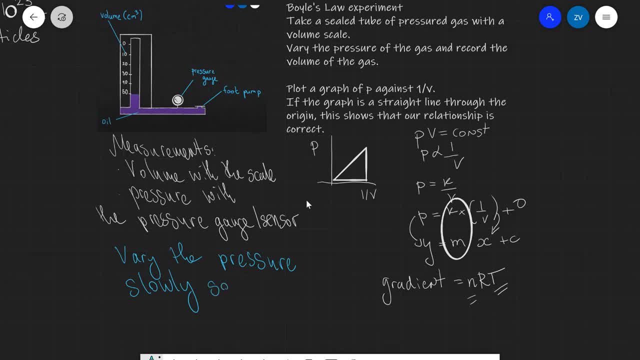 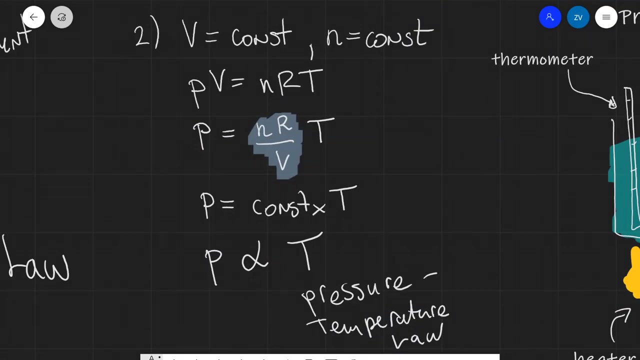 slowly so that the temperature remains constant. for anyone that has pumped up some tires on a bike, for instance, you know that if you vary the, if you pump up the tires quite quickly, that the pump even will get really, really hot really quickly. so we're going to try and keep that temperature constant. now let's 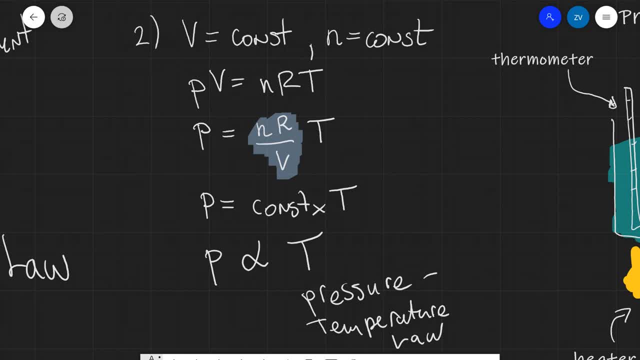 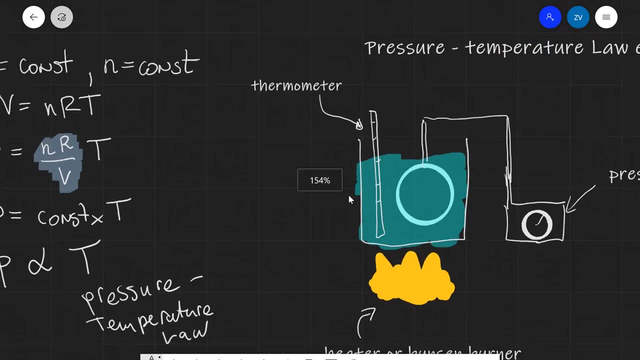 have a look at how we could actually investigate the pressure temperature law. remember that says that pressure is proportional to temperature, which means that the pressure is equal to some constant nR over V multiplied by the temperature. in order to investigate that, we must really need to make sure that the 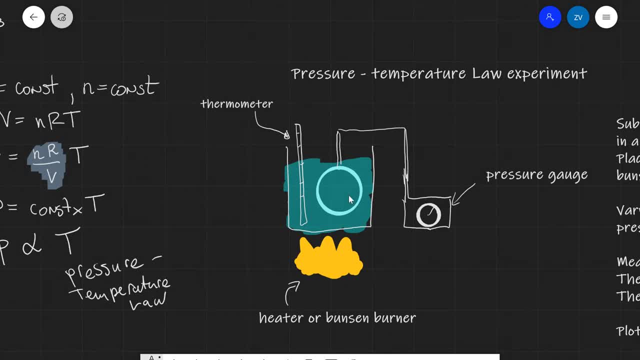 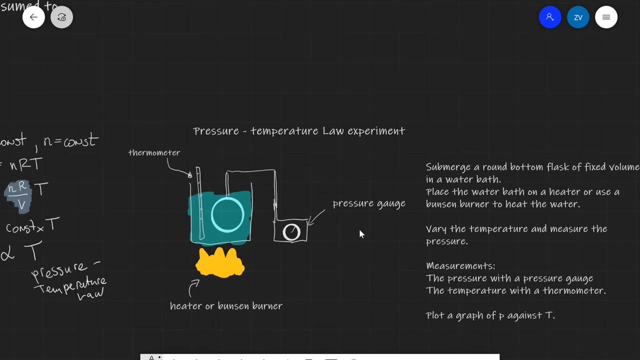 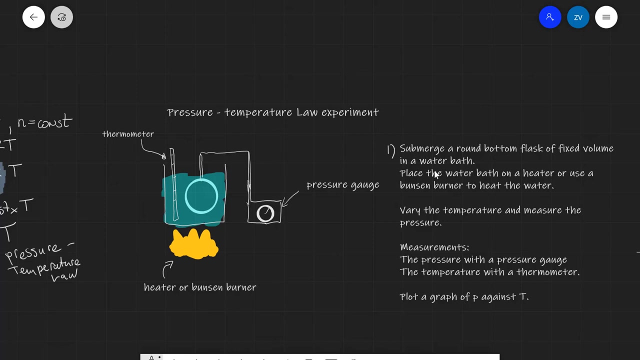 volume of the gas in question is constant and, additionally, the amount of substance is constant. so what we're going to do is we're actually going to use a round bottom sealed flask of a fixed volume and going to submerge that in a water bath. so this will be our first step of the 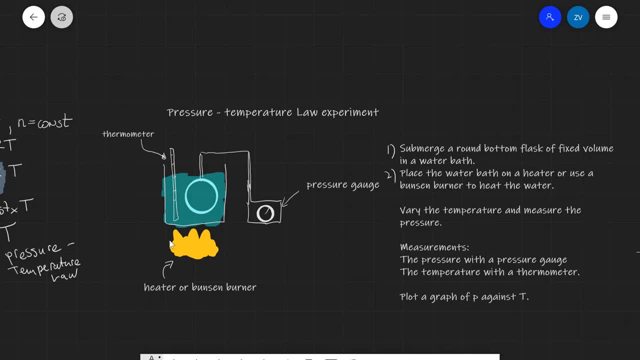 method, then we're going to place that water bath on top of a heater or or a- We could use a Bunsen burner as well- some heat pads to heat up the water, and you can see my artistic impression of the flames over here. Afterwards we're going to vary the temperature and we're going to be measuring the pressure. 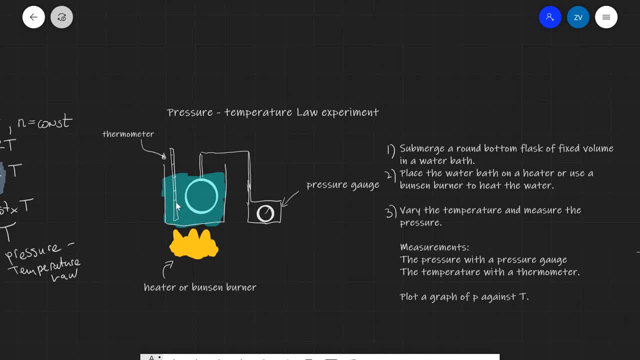 So the water will slowly heat up. so we could start- could even start- with ice at zero degrees Celsius and then slowly, essentially heat up the ice, melt it, make sure it turns into water, and then the water can sort of heat up. We're going to take measurements, regular measurements of the pressure with the pressure gauge and of the temperature with a thermometer. 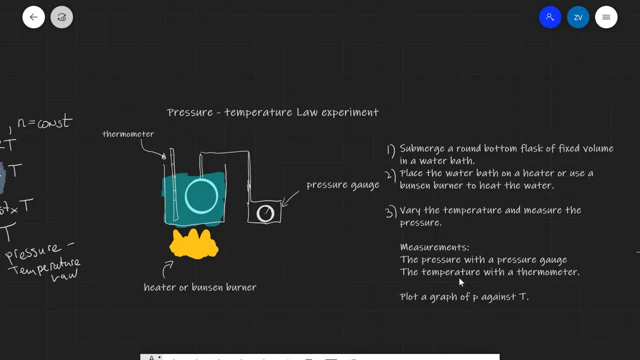 After we have taken a look at the temperature, we're going to take a look at the temperature. After we have taken a look at the temperature, we're going to take a look at the temperature. we're going to plot a graph of P against T. 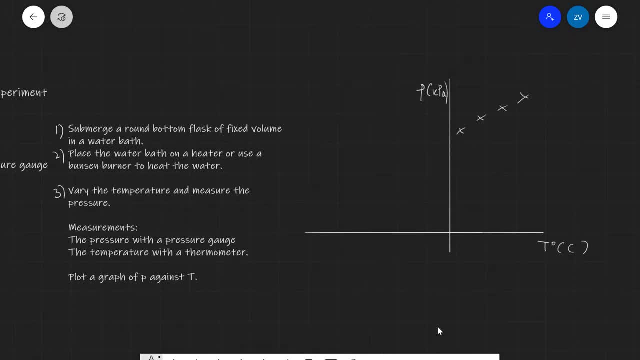 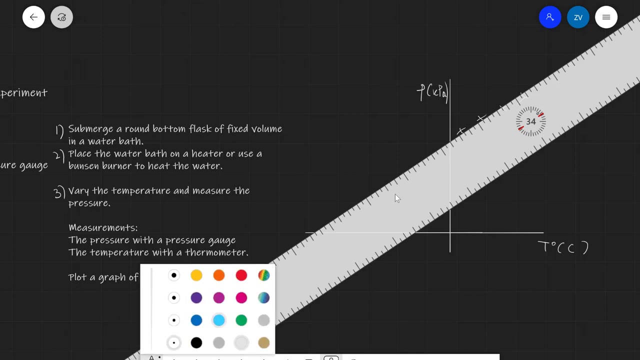 Now our graph will look something like this: So we're going to have our pressure and we're going to have our temperature, and the graph should be a straight line but won't be through the origin. We could actually use, we could actually extrapolate to figure out our absolute zero by drawing the line of best fit and extrapolate. 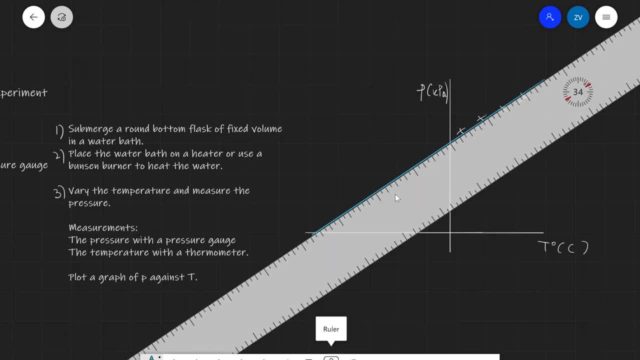 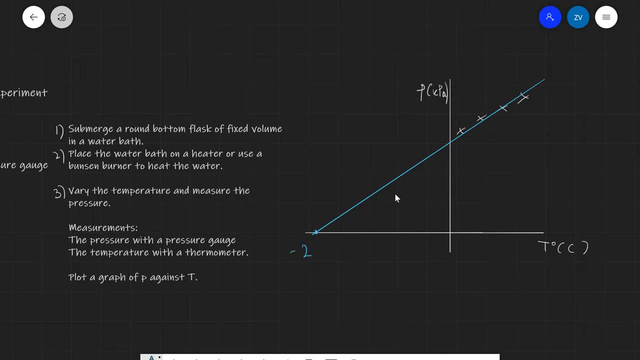 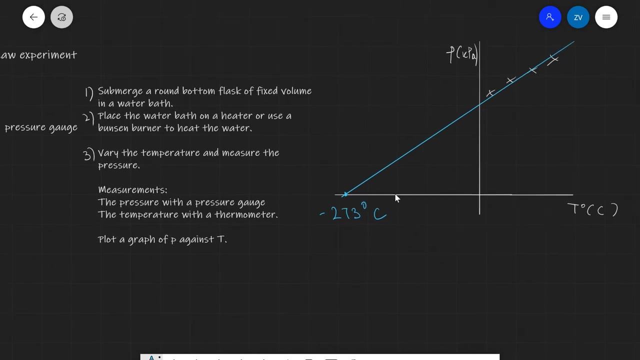 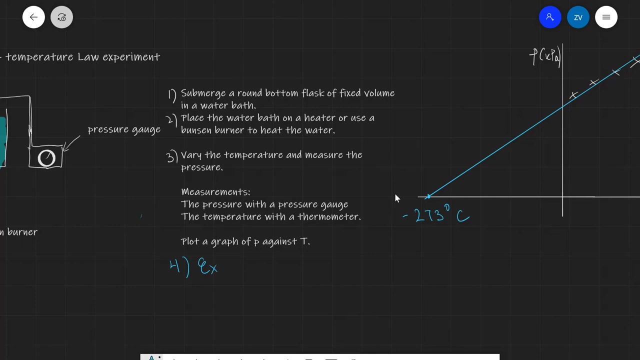 So we keep at. So, um, let's do this, So we're going to extrapolate, to flow, Or um, let's just write this down because this is very important. So let's write it right over here in blue: so we're going to extrapolate. or um, let's just say that we are going to draw a line that is further down from the top, somewhere inside here, and we have to move really, really close to the top. 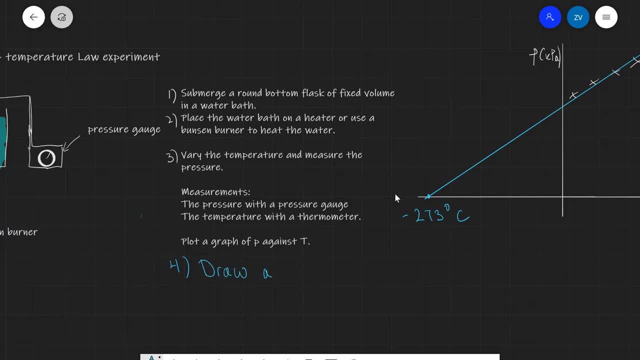 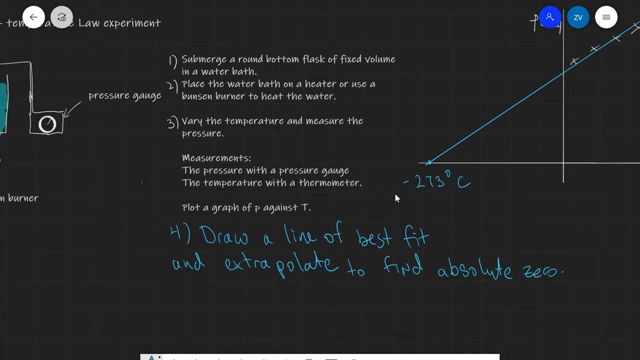 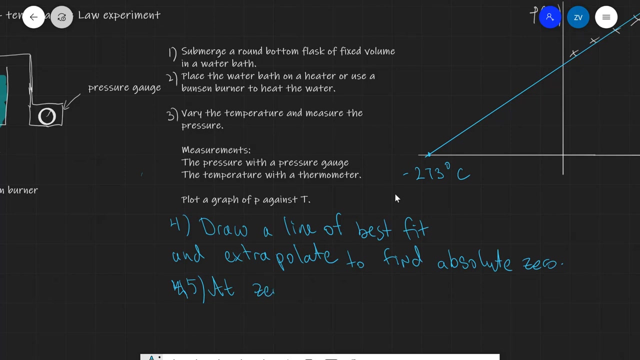 of best fit. so draw a line of best fit and extrapolate to find absolute zero. zero, like so, and at zero pressure. so that's be the fifth point: at zero pressure you'll find absolute zero. now remember, at absolute zero the particles have minimum internal energy, which would mean that their kinetic energy is. 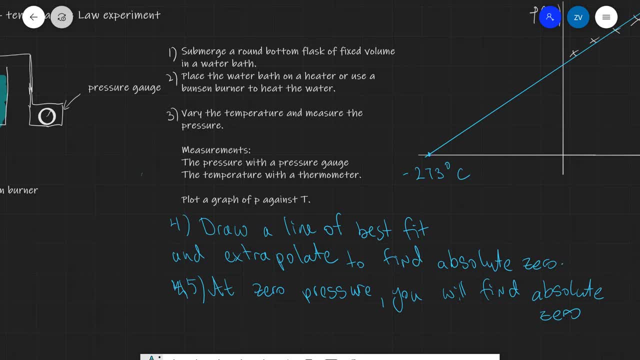 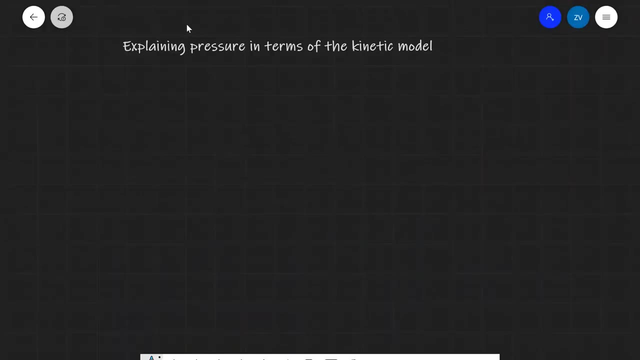 starting to tend towards zero, so they're hardly exerting any force on to the container. there's hardly any change of momentum of the particles as they're colliding, which means it's hardly going to be any pressure on the container so far. we've talked quite a lot about pressure in terms of the kinetic model. 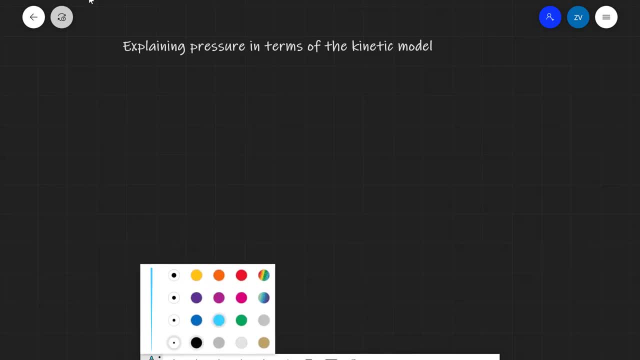 but let's actually explain this using the kinetic model. what actually is pressure? well, let's imagine the side of a container and let's imagine that we have a molecule of gas which is going towards it and the molecule is going to collide with the container. then for 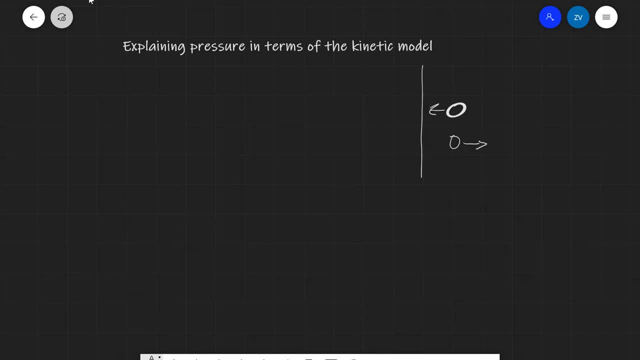 rebound back into the opposite direction. if the initial part of the initial momentum of this particles, and V, the, the final amount of the particle, is going to be MV direction, assuming, assuming that no energy has been lost. so we can just say that this is equal to minus MV. so there's going to be a change of momentum. 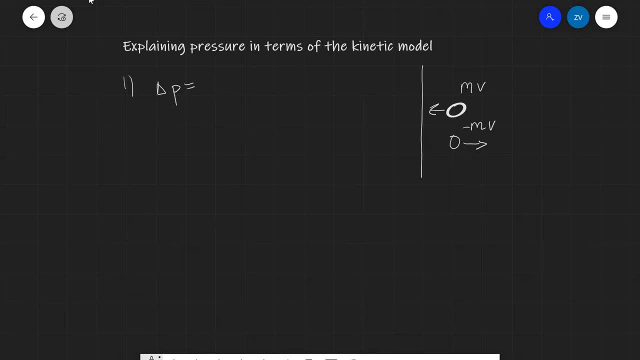 and that change of momentum will be equal to final momentum, which is minus MV, minus the initial momentum, which is MV, which is equal to minus 2 MV. but remember: anytime there's a change of momentum, there is a force that must be acting as well. Newton's second law says: net force acting on an object is: 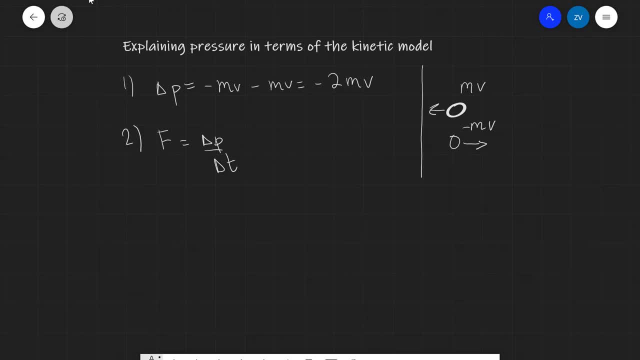 proportional to the rate of change of momentum, so that individual particle is going to experience a force of minus 2 MV divided by Delta T, and the same force will be experienced by the container, but in the opposite direction now, because pressure is equal to force over area in general, if we imagine there's so many of these. 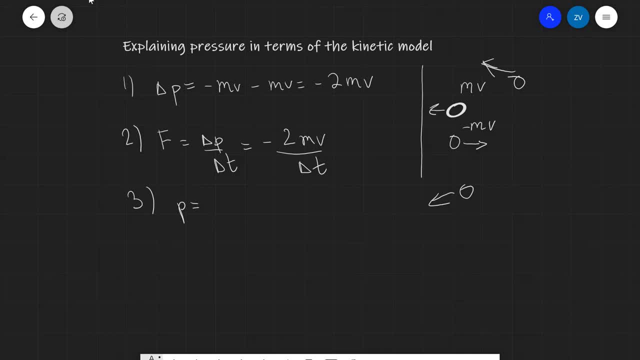 particles which are constantly colliding with, with, with the container. let's say the container is is here across all sides. if we sum all of those forces and divide them by the area, this is what pressure actually is. so it's the sum of all forces, of those could, those collision forces, the particles divided. 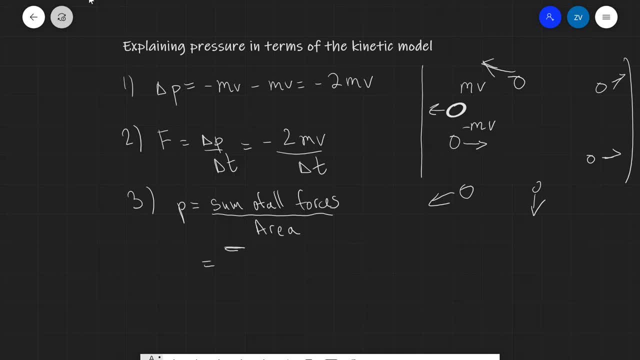 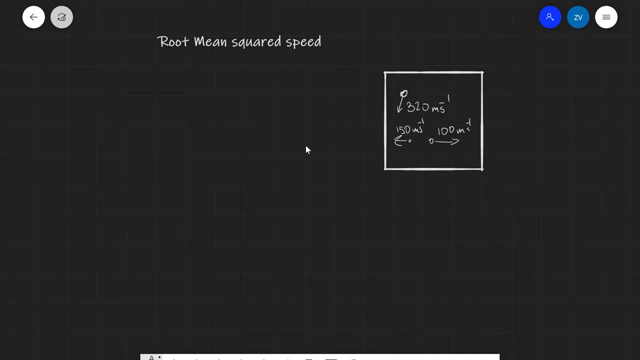 by the area. so let's just write that mathematically as the sum of all the forces divided by the area. this is what pressure actually is on a small scale. okay, now let's talk a little bit about the root mean squared speed. so there's many, many different molecules in a gas, billions and billions of them, and they 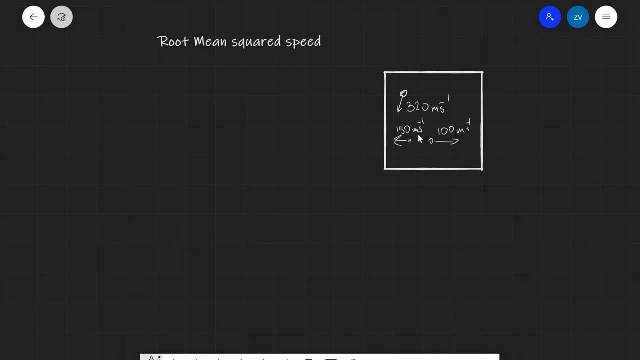 all have different velocities in different directions. so we need another method to have an idea of how much on average, the, the, the speeds of the particle are, and we use the root mean square speed for that. so imagine we have some particles over here. let's say 320 meters per second. one is with 150 in this. 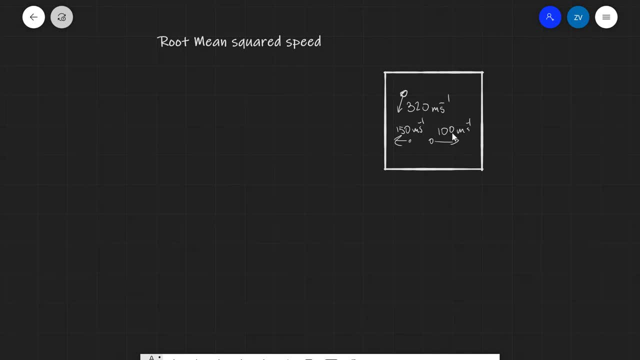 direction and the other one is a hundred meters per second in the opposite direction, then what we need to do would be to first off square the speeds, then afterwards we're going to take the mean and then afterwards we are going to find the square root of our result. okay, well, let's. 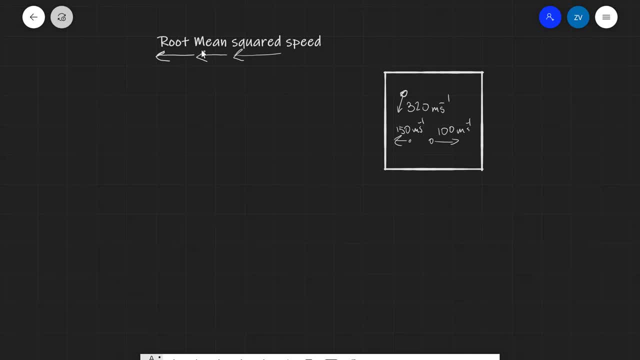 start off first off by squaring them so and then taking the mean. so it's going to be 320 square plus 150 squared plus a hundred squared, and this is only three particles. in our hypothetical scenario we're going to divide the speed by the by 3. so let's do that on the calculator: 320 squared plus 150 squared plus 100 squared divided. 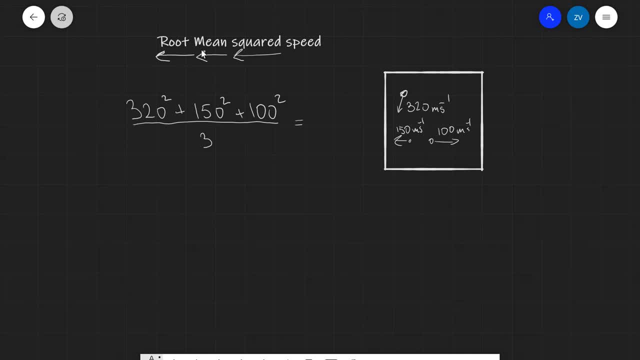 by 3 and that's going to give me approximately- let's just write it down over here- as a 4.4 multiplied. actually, let's just involve a little bit more precision because we're going to be square rooting the answer and i'm going to put it into the appropriate sign of configures right at. 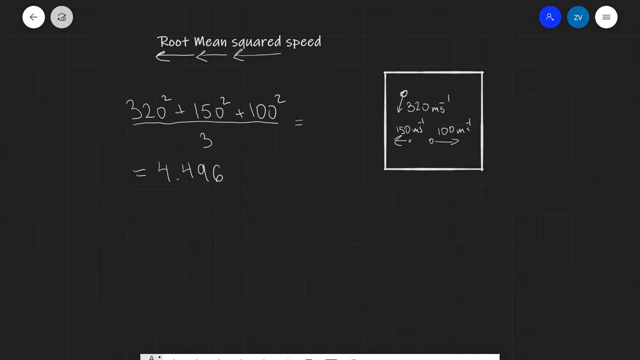 the very end. so it can be 4.4967 times 10 to the power of 4. that's going to be meter squared s to the power of minus 2. okay, well, we have squared speed and we found the mean of the squares. now. 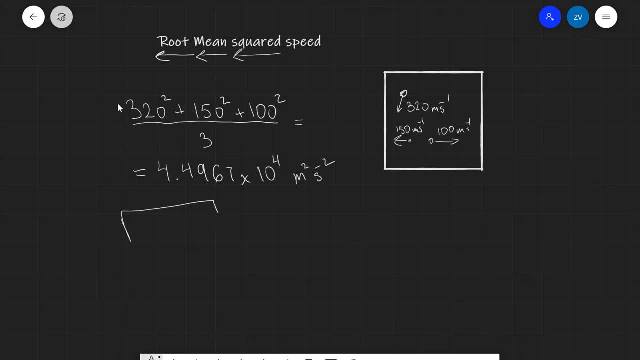 let's just square root our answer. so it'll be the square root of 4.4 point four, nine, six, seven times ten, to the power of four, to get a root mean square speed of approximately 212 meters per second, because we're using up to two significant figures. 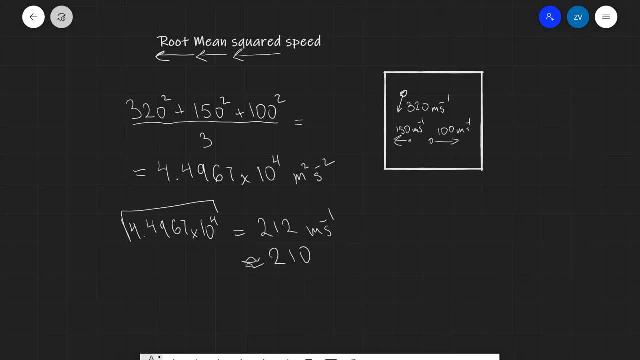 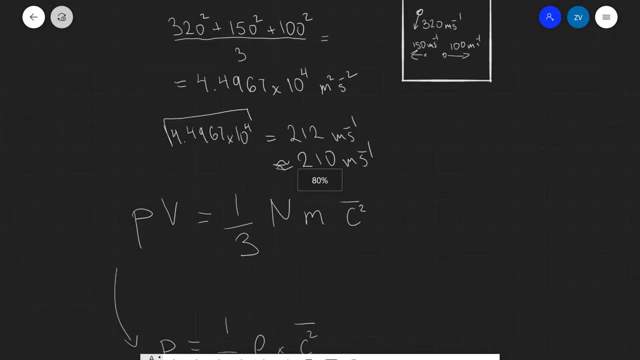 in this. we could also leave that as about 210 meters per second. now, the mean squared speed is really important to know that we're going to be square rooting the answer. so let's just in this equation in particular, which says that the pressure times the volume: 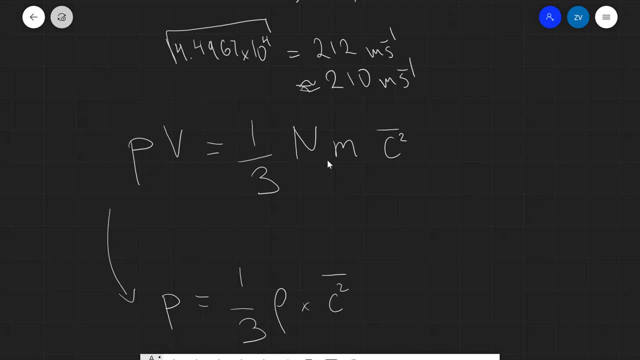 is equal to one third times the number of particles multiplied by the mass and then multiplied by the squared mean speed. Notice, this is not the root mean square speed. If it was, there would be a square root sign here, but there is not. So we've just squared the values and taken the mean of them. A typical exam. 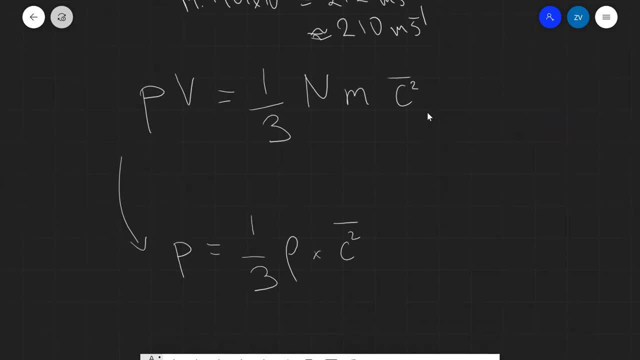 question might ask you to derive that the same equation up here can be written: as the pressure is equal to one third multiplied by the density of the substance times the squared mean speed. Okay, well, how are we going to tackle this? First off, remember, the density is. 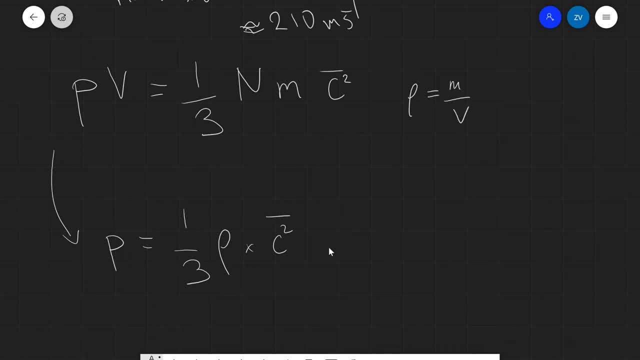 equal to mass over volume. Now the total mass of a patient is equal to the volume of the substance multiplied by the number of particles of the mass over it. So that is the total mass of a patient, the total mass caliber and the unit volume over the force. 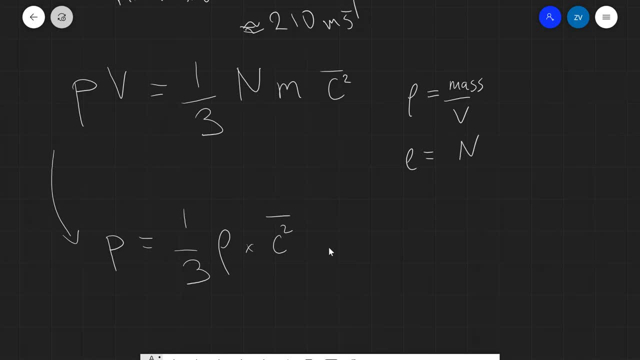 the gas will be equal to the number of particles multiplied by the, by the individual mass of each of them. then we're going to be dividing that by the volume. so let's see how we can proceed. one thing we could do is just rearrange for the volume, then plug that into the original equation so we can say that the 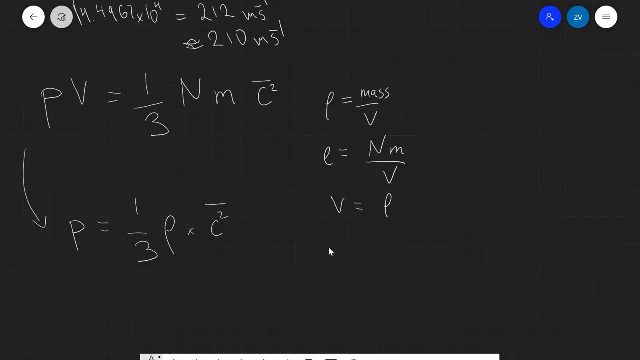 volume will be equal to the density. I mean, of course, that the volume be equal to the number of particles multiplied by the mass divided by the density. okay, so, now that we have V, what I'm going to do is I'm just going to substitute that in 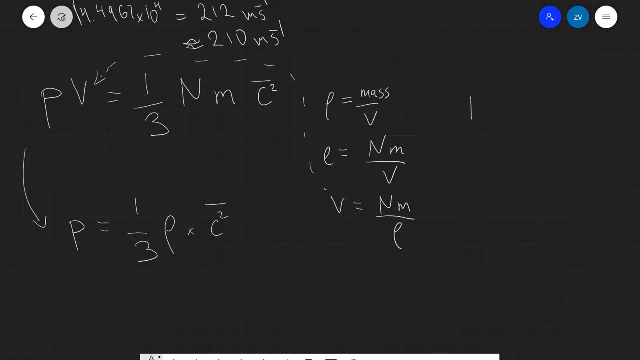 here, and what we're going to get is that P, and rather than times V, I'm going to say times N M divided by the density, is that P, and rather than times V, I'm going to say times N M divided by the density, is equal to a third N M C squared. we're basically there, aren't we? so we can. 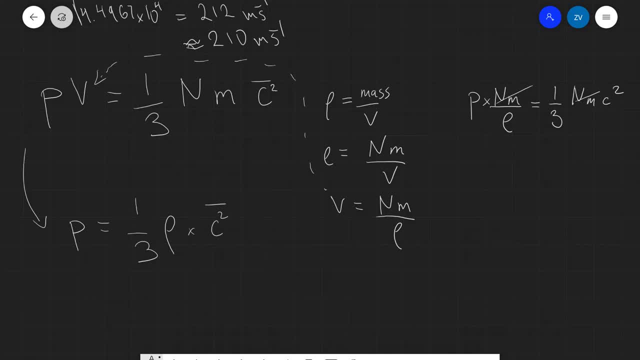 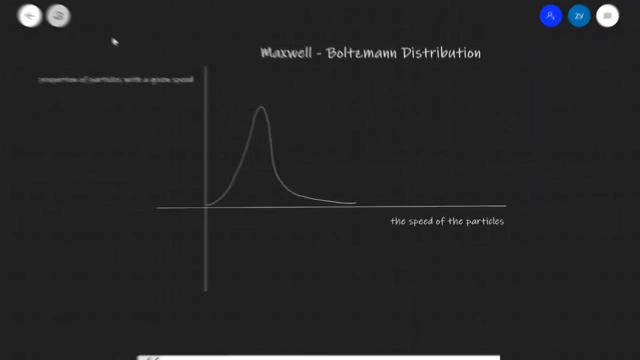 cancel out N, M on either side, and what we're going to get is that the pressure is equal to a third times the density. times the squared mean speed. okay, so up next is the Maxwell Boltzmann distribution we've been talking about when we've been revising about the speed of the 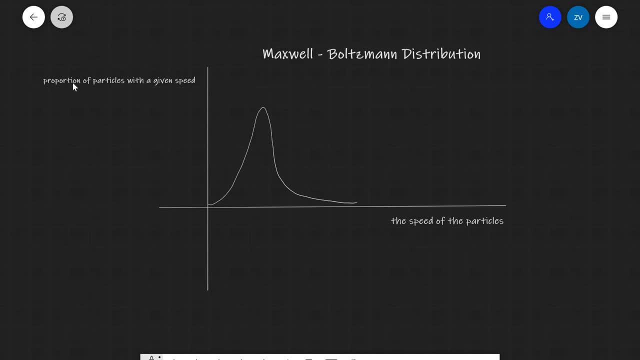 particles. the Maxwell Boltzmann distribution is a plot of the proportion of particles with a given speed against the speed of the particles. so we can see that quite few of the particles, a relatively small proportion, have low speeds and could just write this down so we can say that. 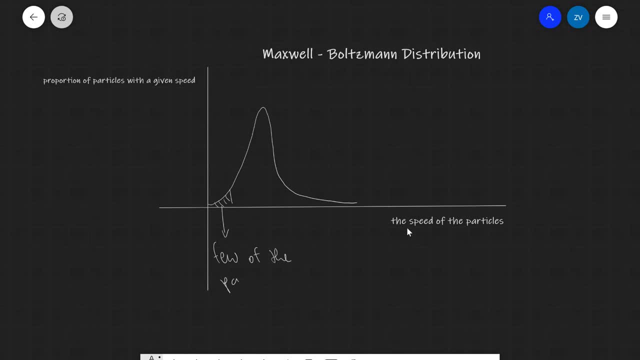 few of the particles have low speeds, low speeds. however, the vast majority of the particles will have moderate speeds, and this will be this region over here. maybe I can just sort of highlight it like. so it will be just this region over here, with where the vast majority of the 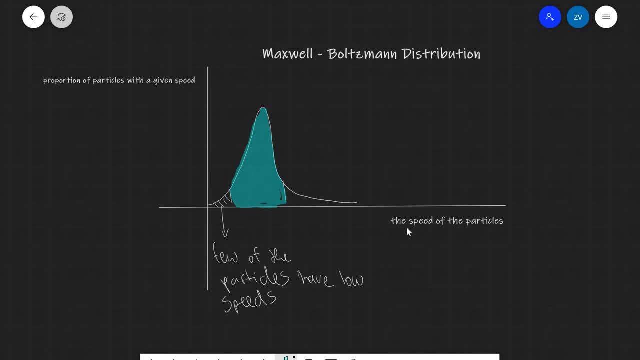 particles are. you can see that those are the particles with the, with the greatest proportion in terms of numbers. so we can say that most of the particles, most of the particles, have moderate, moderate speeds. we can see that here, that the speed is still not quite high for a very, very small proportion of the particles. 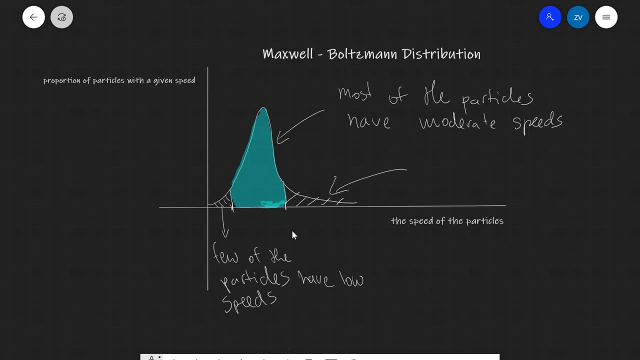 will have some very high speeds, and then we can also say that a few of the particles will have moderate speeds, and then we can also say that a few of the particles will have very high speeds. now what will happen to this curve if the temperature changes? so let me draw with a different color what we 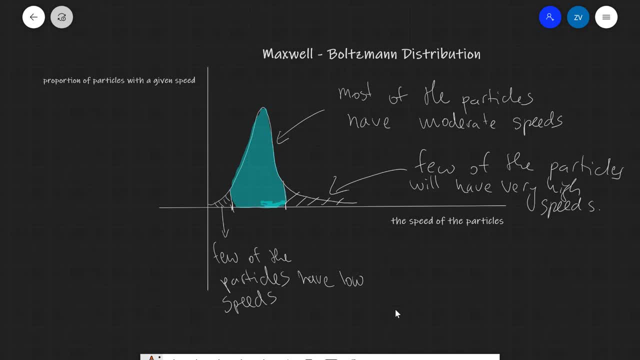 expect to see. if we increase the temperature first off, the curve will become flatter and more of the particles are going to end up having higher speeds. so the graph will suddenly appear to look something like this. so let's see if I can use a larger highlighter. so it will. 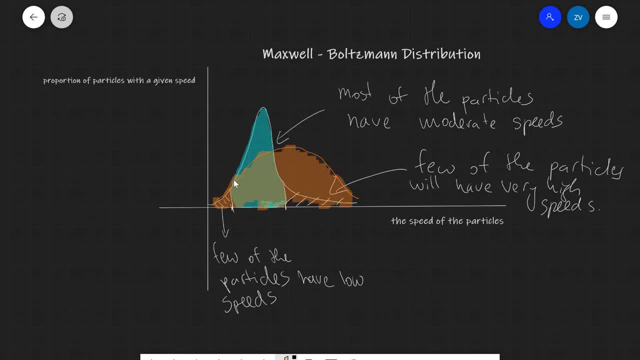 look something like this, in which more of the particles are going to have larger speeds. so just write that here. so this orange graph here will look a little bit represents what would happen if we increase the temperature. So this is a graph for a higher temperature, where once again there's a greater 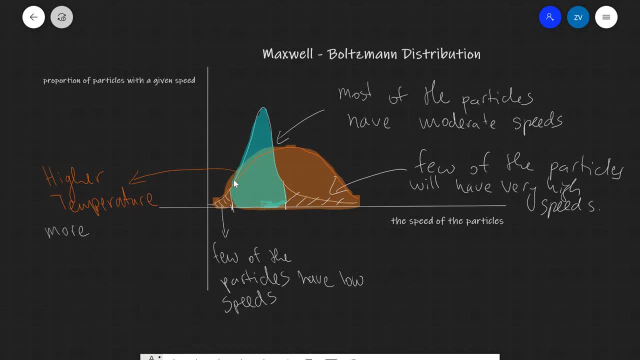 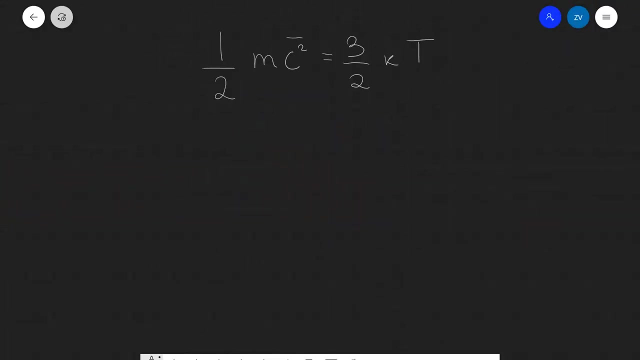 proportion, or there's more particles at higher speeds. So there seems to be a link between how quickly a particle is going and then what the temperature is. Let's have a look at that link. The link is to be found within this extremely important equation, which really tells us what temperature. 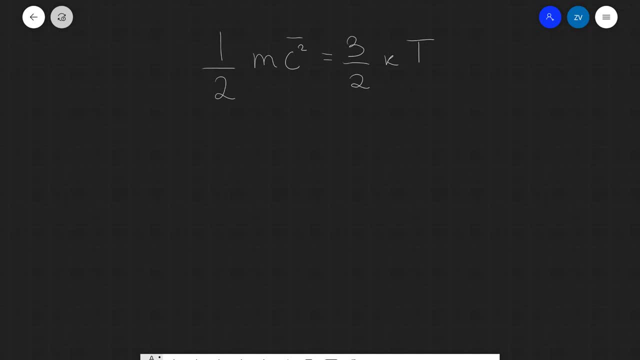 actually is, And that is that the mean kinetic energy a half m c squared, where c squared with a bar on top signifies, as we're taking the mean squared speed is equal to three halves times K, which is Boltzmann's constant constant 1.38. 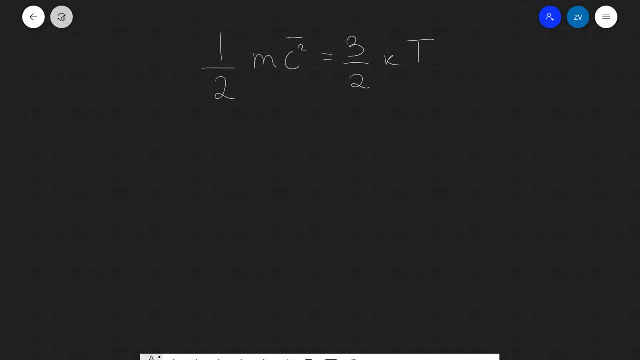 times 10 to the power minus 23 times the temperature in Kelvin. Just please remember that this over here is the temperature in Kelvin, this over here is Boltzmann's constant. so Boltzmann's constant, given you form the booklet, but 1.38 times 10 to the power minus 23, this is just the halves representing the degrees of 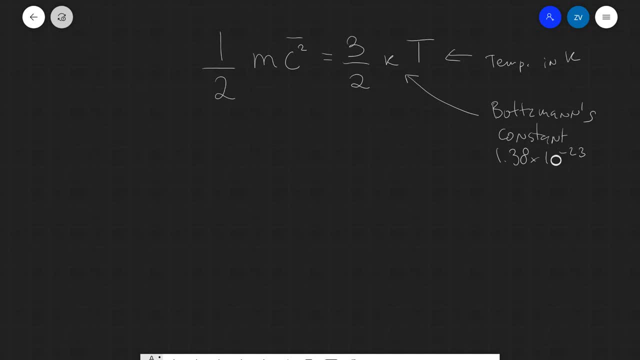 freedom. This is something you only sort of worry about if you study physics at university. C squared is the squared squared mean speed and M is the mass of a particle of the gas. So this means that, for instance, if you know the mass of an air particle, you 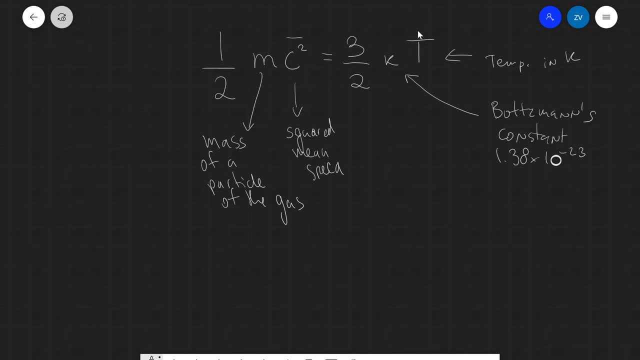 will know that, at a given temperature, the speed should be something which you can actually calculate, to be able to calculate the squared mean speed or the root mean square speed of a particle of air at a given temperature, which is really, really exciting. Now, how can we actually come up with? how do we actually come up? 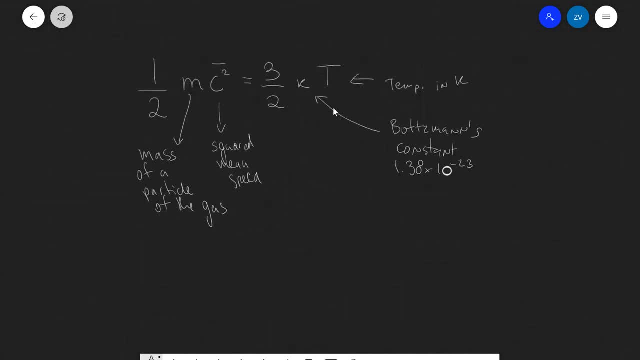 with this equation. how can we derive this equation? and this is something that we need to know for the exam. So let's practice it. So the way to derive this expression is: first off, let's look at a starting point. So anytime we're deriving something in 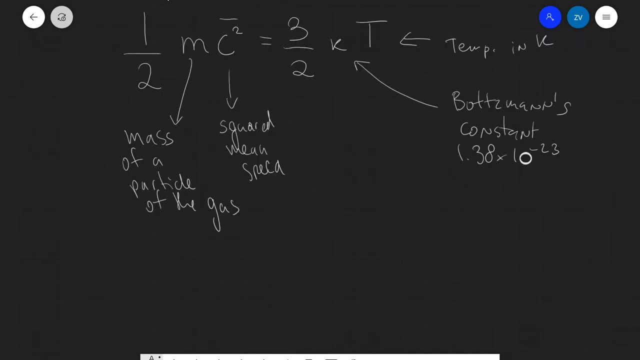 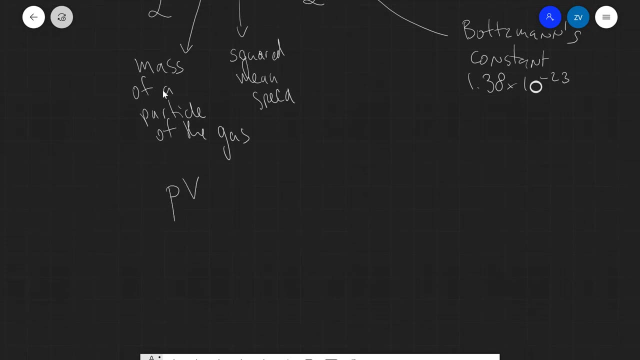 physics. we need to look at some other equations and then finally come up with this equation. so the derivation of this one is relatively straightforward. We have two equations in our formula booklet. One is a, PV, The other one is a. is equal to 1 third multiplied by the number of particles, multiplied by the mass, multiplied by. 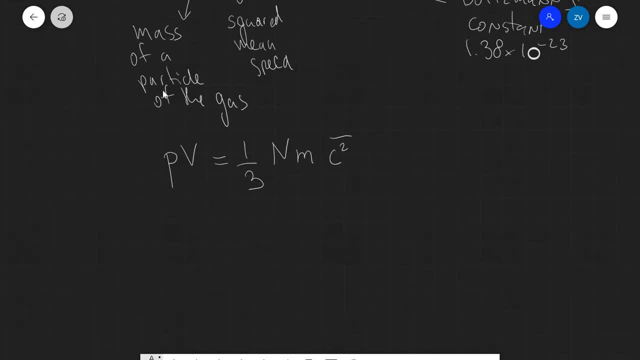 c squared with a bar on top. the other one is that pv is equal to n, where n is the number of particles. again k is Boltzmann's constant and t is our temperature in kelvin. well, hang on a minute. this equation is for pv and this equation is for pv, so we can just set those equal to one another. 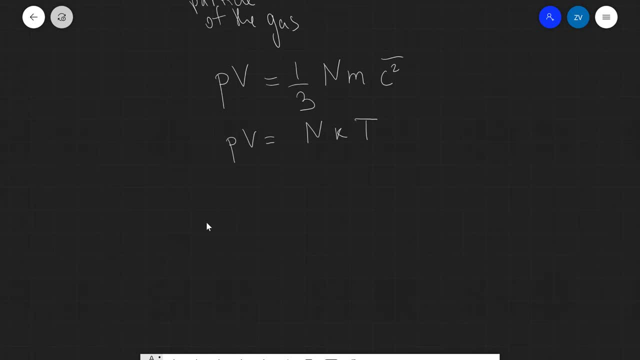 so what we could really easily say is that one third n m c squared is equal to n k t. okay, so now we can cancel out the n's like so, and what we're left with is a third m c squared with a bar on top is equal to k times t. now let's do a little mathematical. 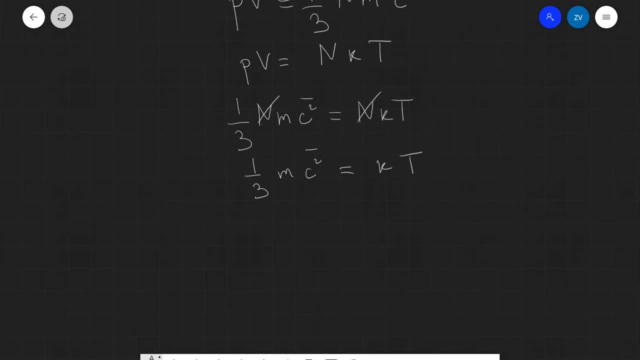 trick here, so we're going to do a little mathematical trick here. so we're going to do a little mathematical trick, so we could represent a third, because in the equations we're applying, that we're trying to prove, there's a factor of three over two. but we could just represent this third as simply. 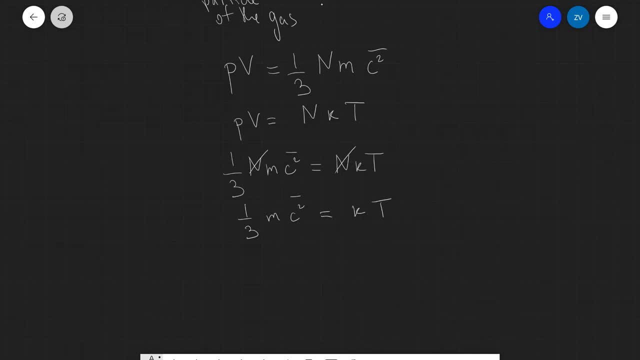 as simply two over thirds, times one over two, because the twos would would just cancel each other out and what we're left with is one over one over two, so we could just represent a third over three. so m c squared, that's equal to k times t. we're basically there, so what we're going to get. 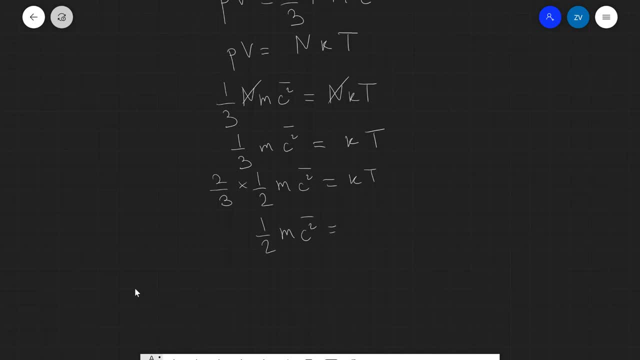 is a half m c squared, which is equal to three halves k t, and we have successfully proven our equation. okay, now that we have done this, we've derived this equation- let's see whether we can apply it to a problem. so we know: the molar mass of area is 29 grams per mole. estimate how. 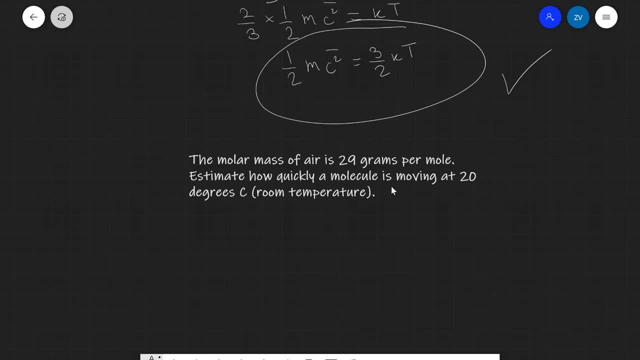 quickly. a molecule is moving at 20 degrees c room temperature. as soon as i see this in question, what i will do is just really quickly, you know, convert that to kelvin, because my equation will only work in kelvin. so we need to add 273, so this will be equal to 293 kelvin. okay, well, we're going to need. 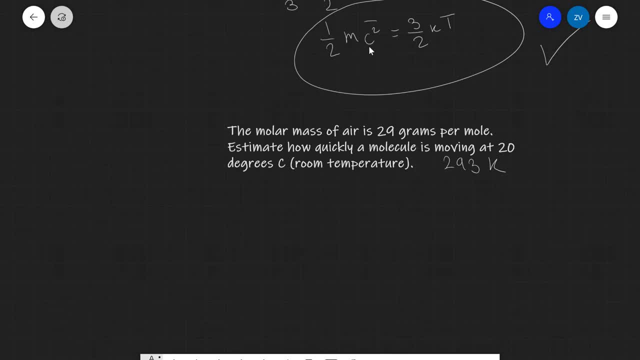 to know the mass of a single particle, to estimate c squared from there, because we know the temperature, we know boltzmann's constant and the only thing that we don't know is m. however, we have the number of grams per mole, so that's going to be 0.029 kilograms per mole. however, remember one mole is. 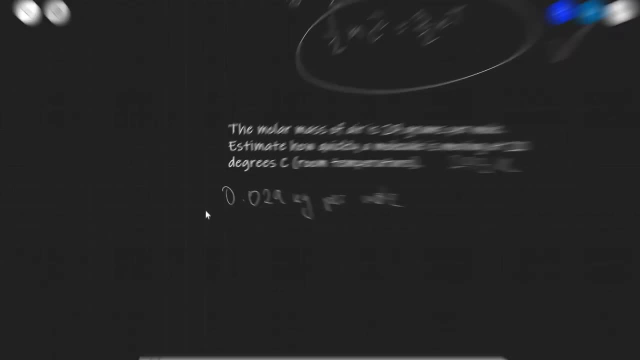 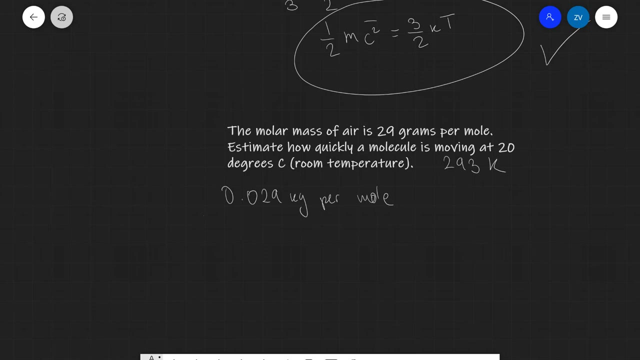 avogadro's number 6.02 times 10 to the power of 23. so if we just divide them, okay, so if one mole weighs 29 grams, then one single particle will weigh 29 kilograms per mole. so that's going to be 0.029 divided by 6.02. so 6.02 times 10 to the power of 23, which is going to give us about 4.8. 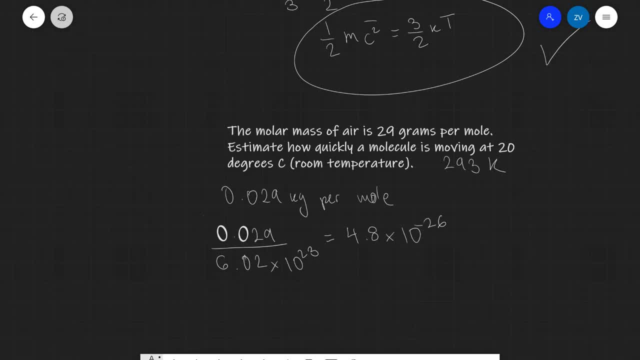 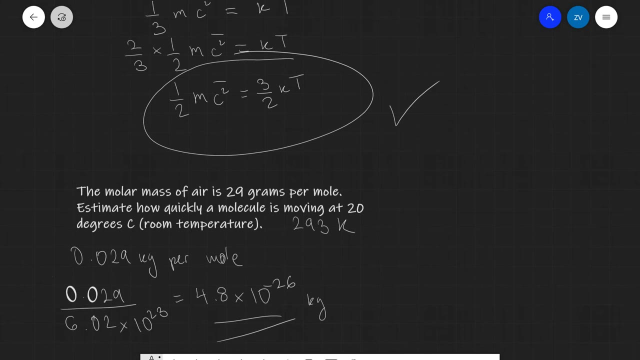 times 10 to the power of minus 26 kilograms. so we're expecting quite a small number, which is which is totally, totally fine. so what exactly what we would expect? okay, so, now that we have the mass, what we can do is estimate the. we could estimate the speed squared, so so let's do that.